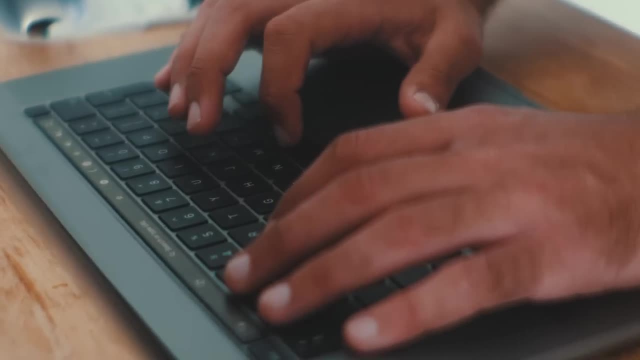 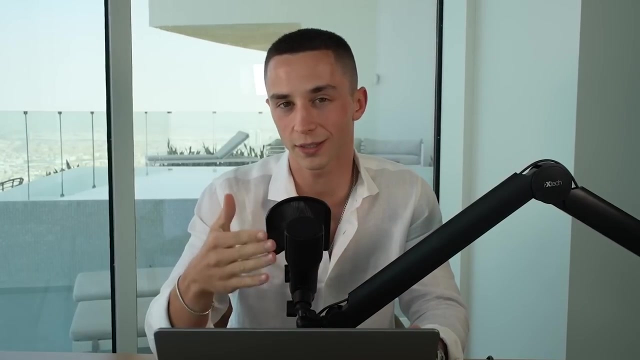 for anyone looking to add this foundational skill of prompt engineering to their toolkit so they can access more opportunities with an AI. So what is prompt engineering? In plain English, prompting is the process of instructing an AI to do a task. We tell the AI, for example, GPT-3,. 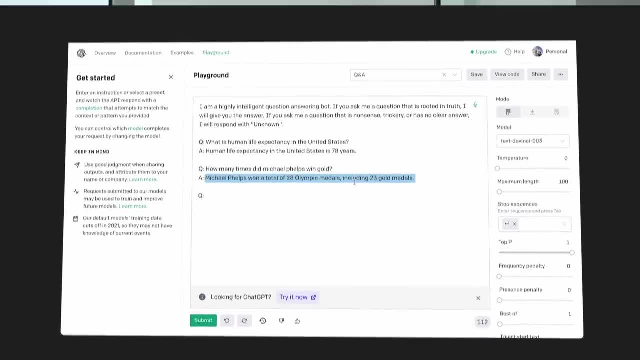 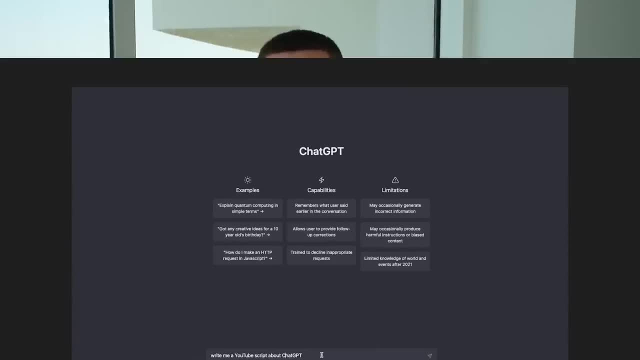 a set of instructions and it performs the task based on those instructions. Prompts can vary in complexity, from a phrase to a question to multiple paragraphs worth of text. I'm sure you've all played around with ChatGPT- The text that you provide in that dialog box. 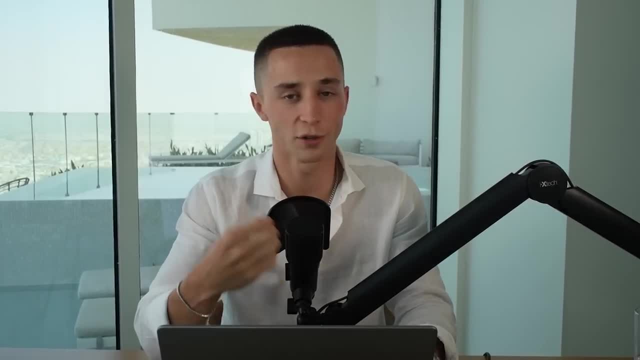 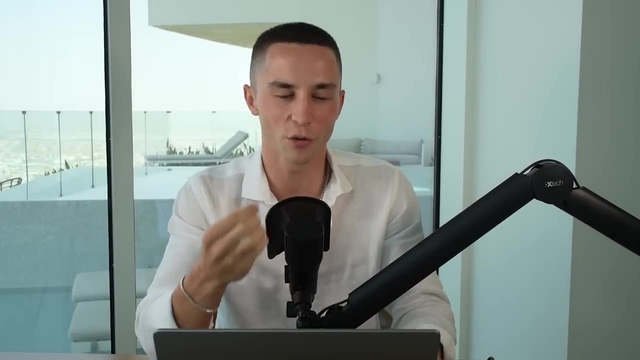 is your prompt. However, most of the value created through prompting is not the same as the value created through prompting. The value created through prompting is not done with ChatGPT. More on this later. The reason prompt engineering, or more simply put, how you construct your prompts, is so important and so valuable is 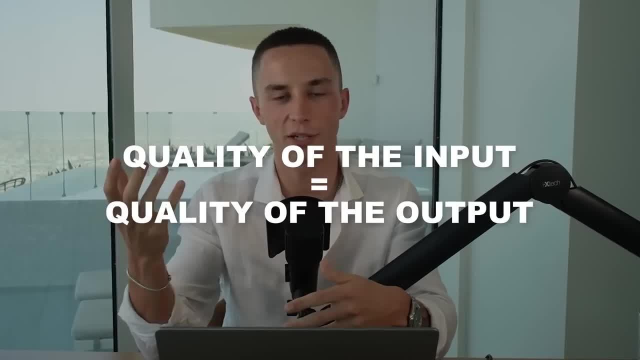 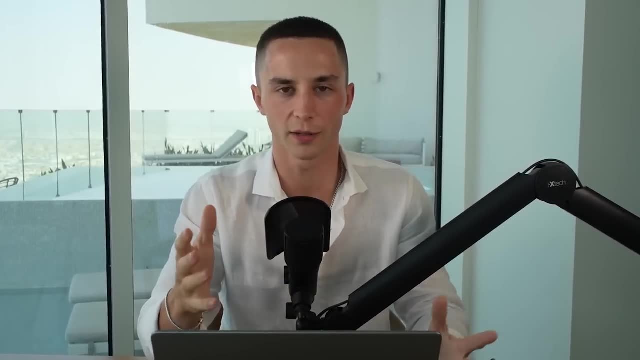 because of a concept called garbage in garbage out. Essentially, the quality of your input determines the quality of your output. When you have large language models like GPT-3 that are massive and are just a soup of data, your ability to write great prompts directly determines your 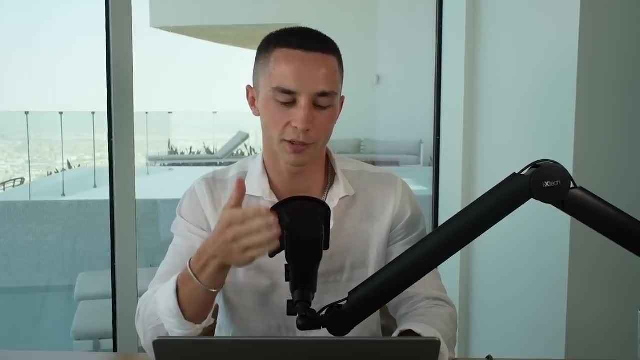 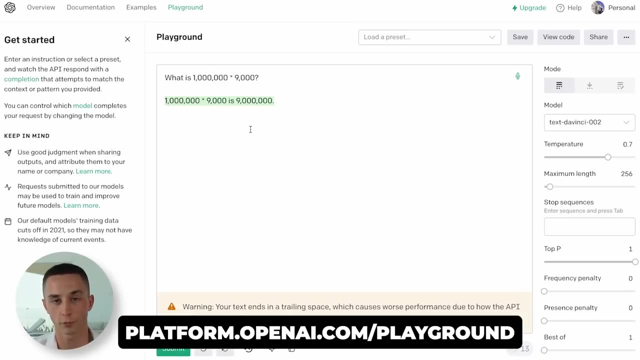 ability to extract value from them. The importance of prompt engineering can be illustrated with a simple example here in OpenAI's Playground. Here on screen, we have a basic master math equation and if I submit that, you'll see that it actually comes back with an incorrect. 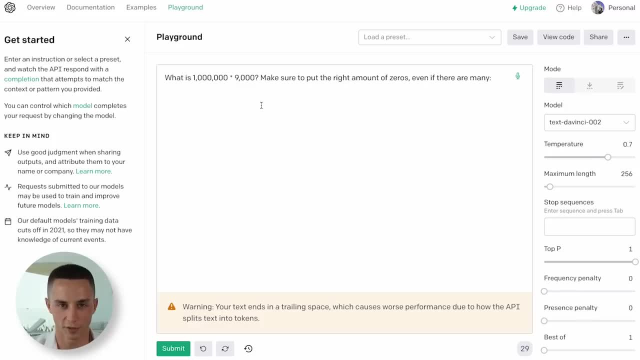 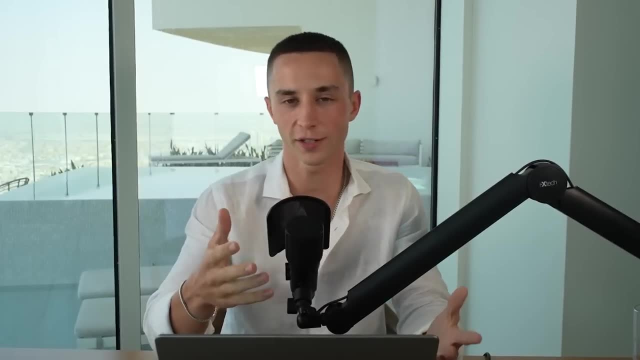 answer. This simple error can easily be fixed with a little bit of prompt engineering. Here I've added: make sure to put the right amount of zeros, even if there are many, And just like that we have the correct answer of 9 billion, As you can see, changing your prompting, just a. 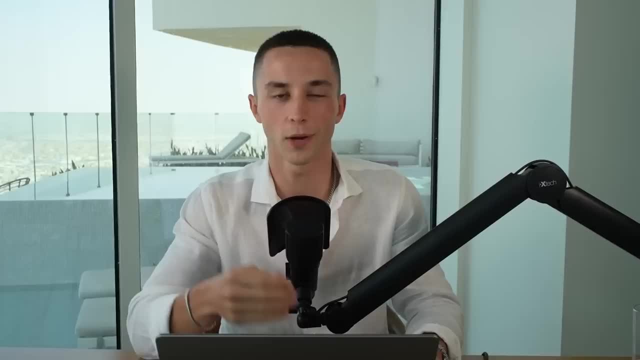 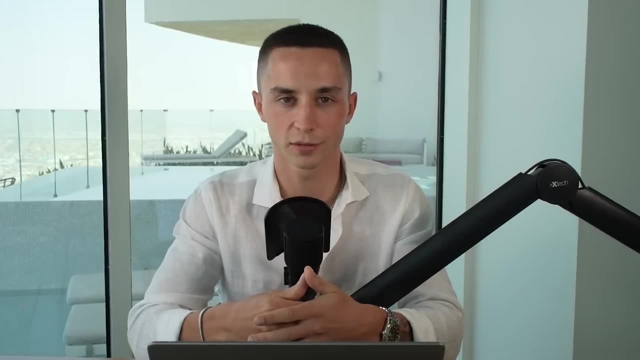 little bit can have drastic effects on having a correct or incorrect answer. While extremely obvious on simple math tasks like this, these slight prompt differences can have an enormous effect on more complex tasks. All this begs the question: how can we make prompts that yield optimal? 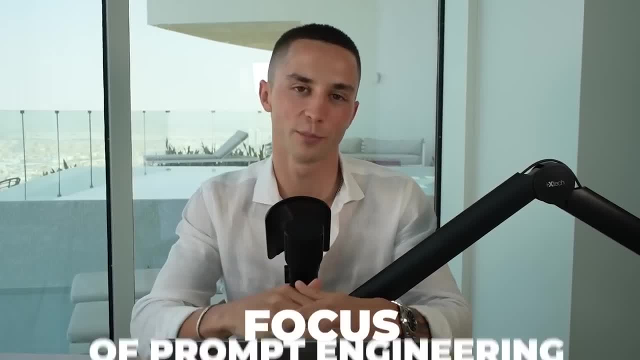 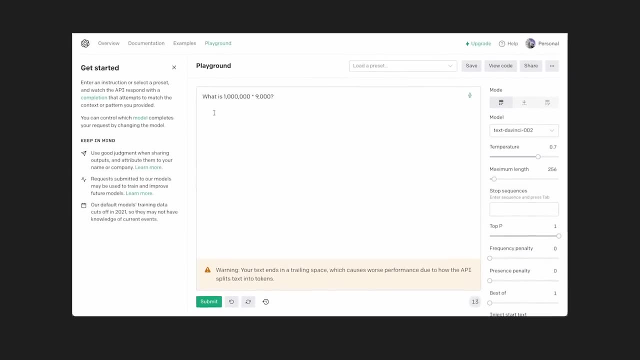 results on any task. This question is the core focus of prompt engineering. Within this video, we will be using the OpenAI Playground for our prompting. It is crucial to understand that the Playground is not the same as ChatGPT, If you're unfamiliar with the Playground. 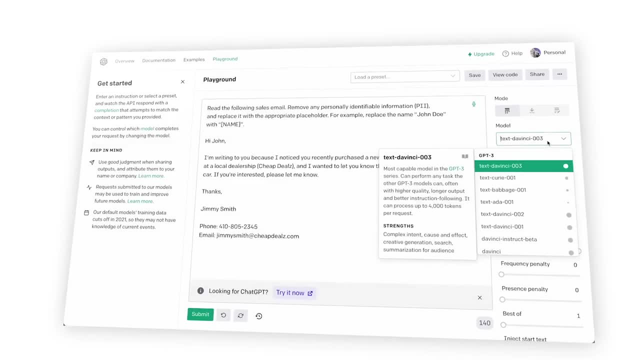 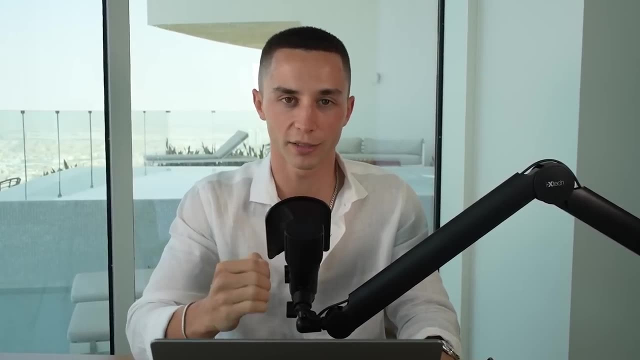 it provides us with a flexible platform that we can interact with all of the OpenAI suite of products in their natural state, And by natural state I mean the form that we get access to them through the OpenAI APIs. This is important to understand because anything 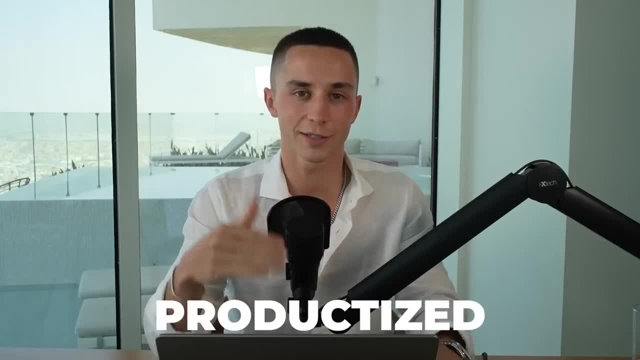 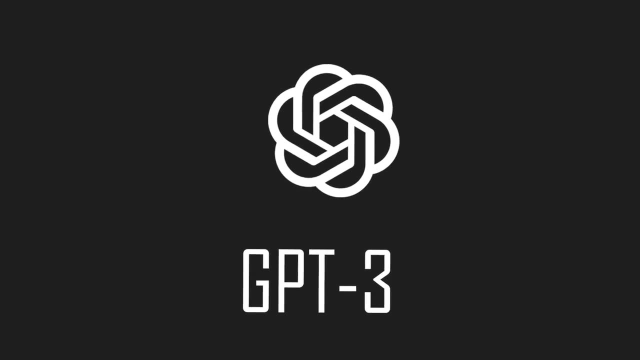 that you can achieve within the Playground can then be scaled and then productized in salt. More on that later. If you didn't know, ChatGPT is actually an application that OpenAI has built on top of the GPT-3 model that we're going to be accessing through the Playground. 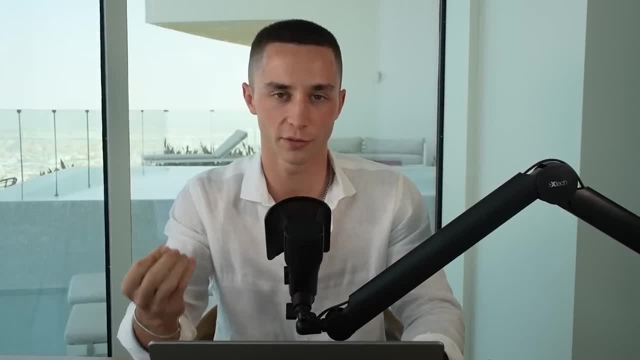 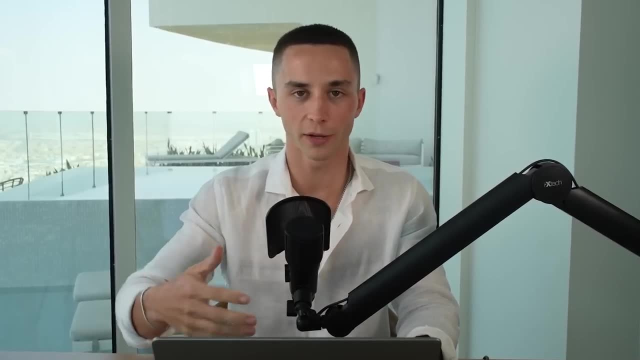 The difference is that OpenAI has significantly changed GPT-3 in order to make ChatGPT, through reinforcement, learning and fine-tuning and a bunch of other fun stuff. Long story short: ChatGPT may be fun and valuable in its own right, but if you're looking to create value and build, 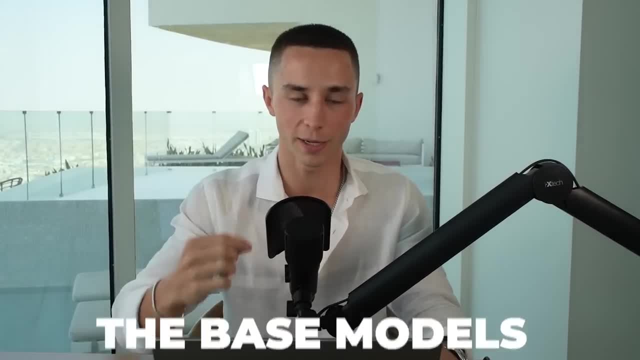 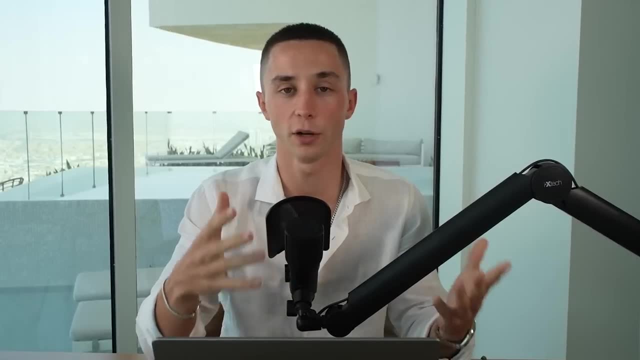 scalable business. on top of these models, you need to be learning how to engineer the base models in their natural state. This is because these base level models are the only things that we can get access to through the APIs currently and therefore the only things that 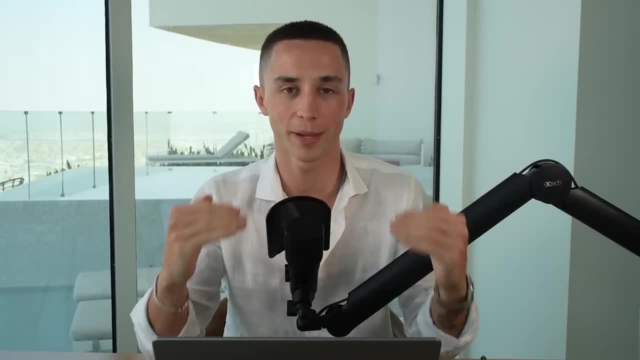 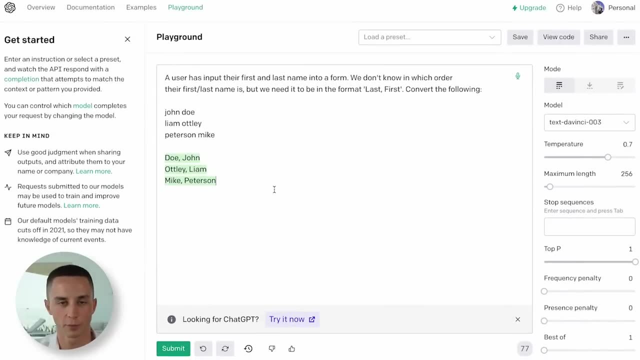 we can build businesses on top of. Therefore, learning how to engineer prompts for the base models through the Playground is going to be the focus of this video. Enough talking, let's jump into the Playground and start prompting. Here we have on screen a very simple prompt that 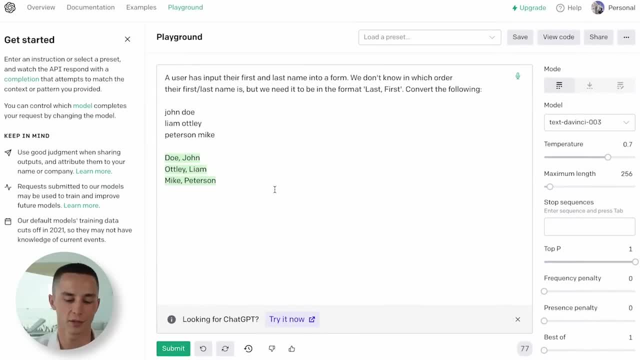 uses the power of large language models like GPT-3 and its understanding of language to convert a mixed bag of first and last names and then order them in last first order. Here you can see I've given John Doe, Liam Otley, Peterson, Mike, and then it's going to output this in last first formatting. 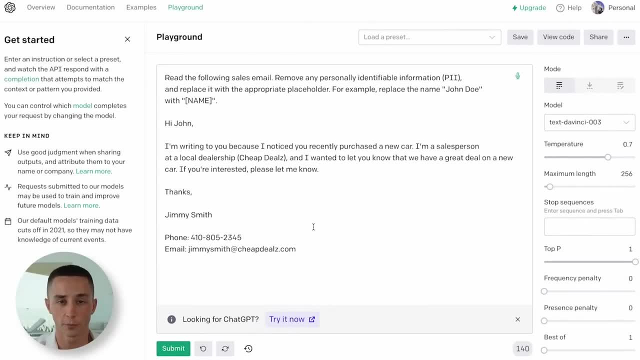 Next up, we have a carefully crafted prompt that allows us to remove personal information from an email. The prompt says: read the following: sales email: remove any personally identifiable information and replace it with the appropriate placeholder. For example, replace the name John Doe with name, and then we have pasted in a sales email example If: 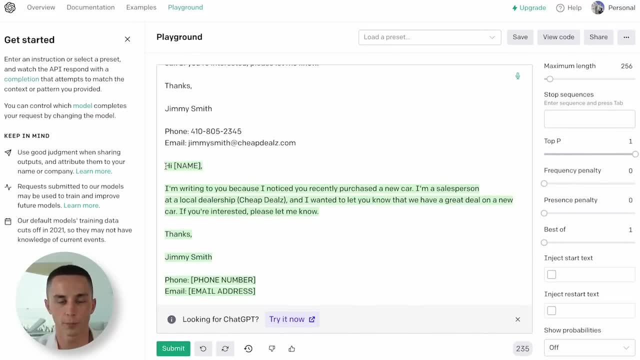 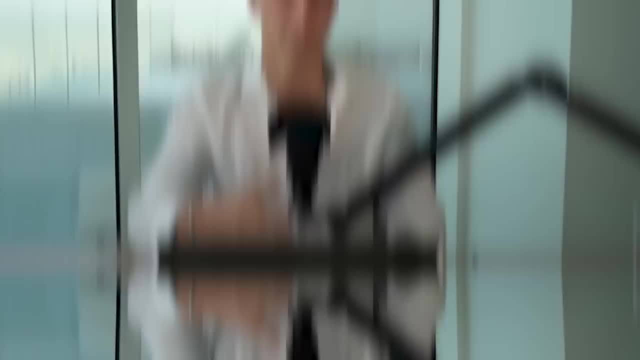 we submit this, the response we get back is the same email with all of the personal information removed. It says hi name, so it's removed the name, and it's also known to remove the phone number and email address as well. Being able to achieve this result within the Playground means. 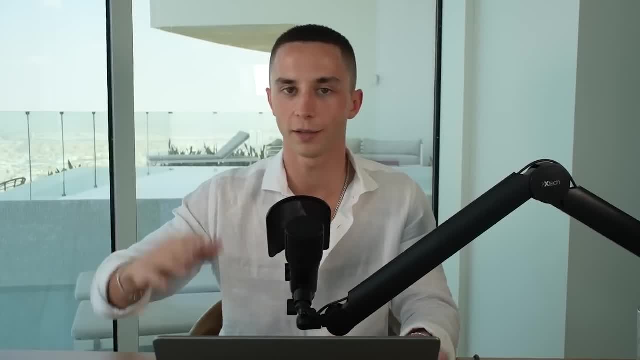 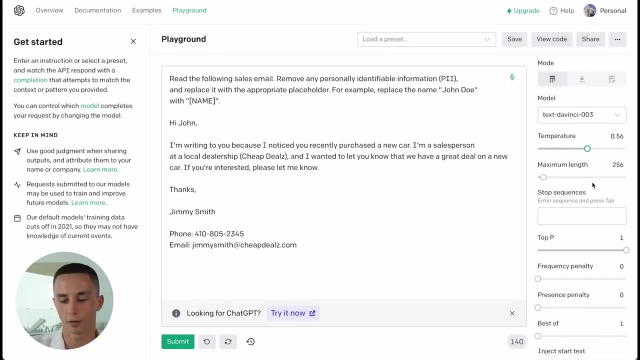 we can then take this exact same prompt and apply it to a larger scale and run it through your agency or something and get these exact same results done en masse. While we're here, I'll give you a rundown of the important settings that you can play around with in the sidebar. First and 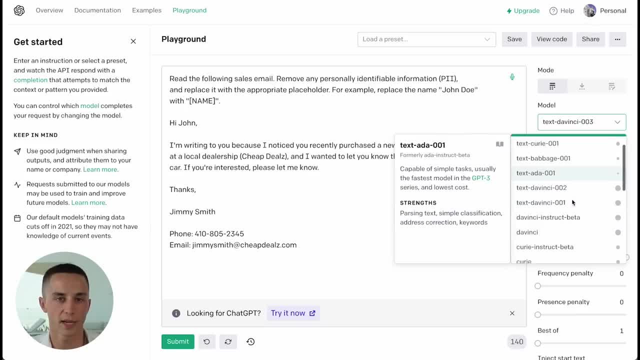 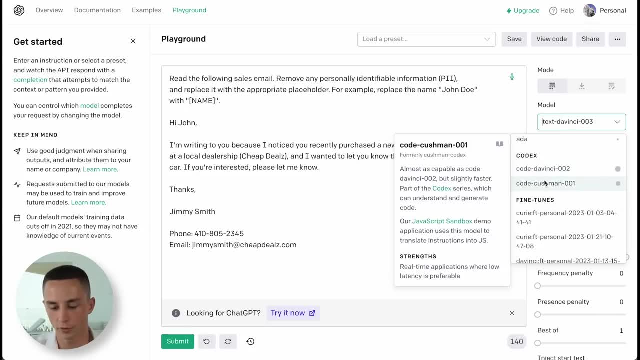 probably most importantly, you can change the model that you're using to interact with. OpenAI has a ton of different models for different purposes. For example, we have code related models here which are more capable of understanding code. We have some of my fine tunes from my 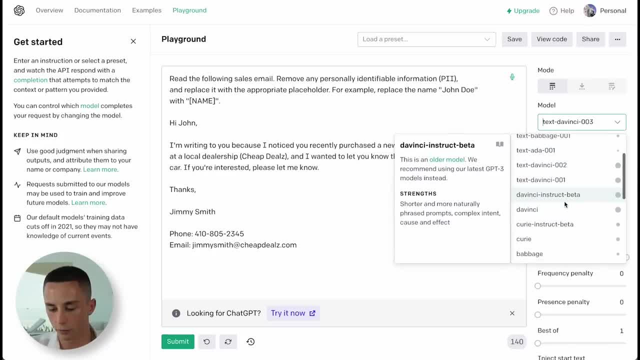 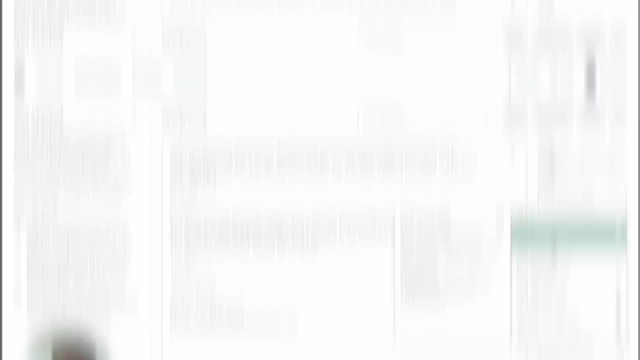 personal account. and then we have different versions of DaVinci Ada, all these different ones that if you look here, it will tell you a little bit of a blurb about what each of these things do and what it's good at. You may be thinking: why would I not just use the best one, which is DaVinci 3 at? 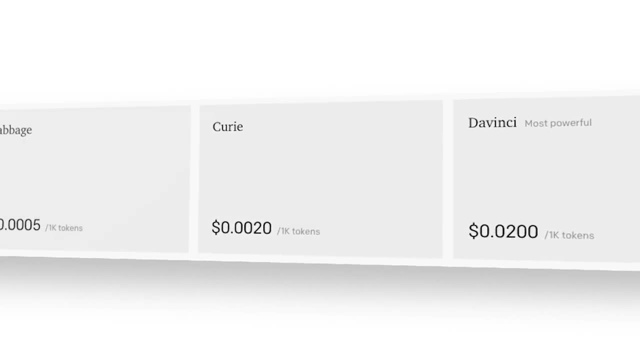 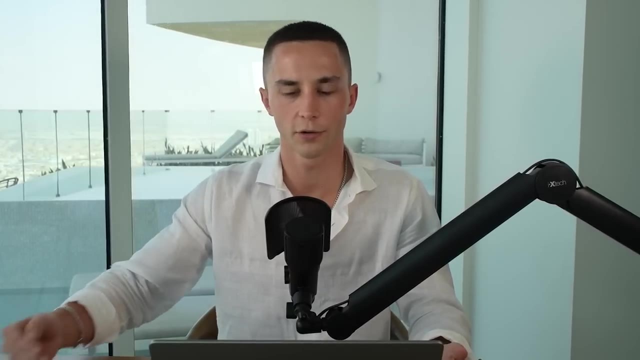 the current time. This is because the pricing for each of these models is actually different. If you want to use these models for a very basic pattern recognition task, you shouldn't be paying more and using the top model, DaVinci 3.. You could be using Curie or Ada or something much lower that. 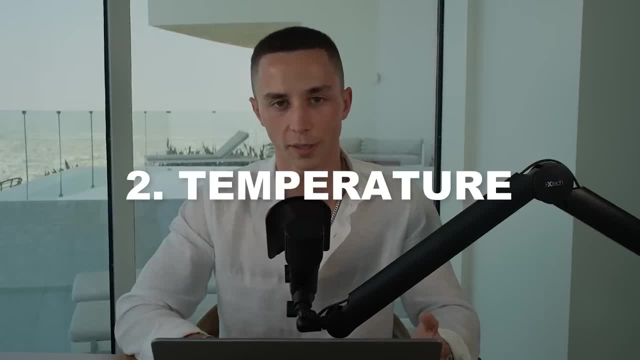 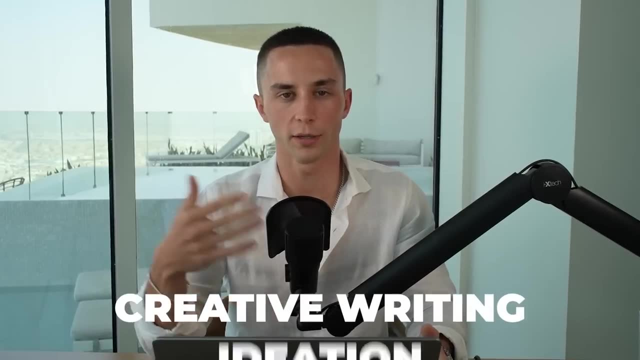 does what you need and nothing you don't. The next and second most important thing you can play around with is the temperature. The temperature setting is crucial because it determines the performance of the model. Some tasks, like creative writing or ideation, would perform better if you 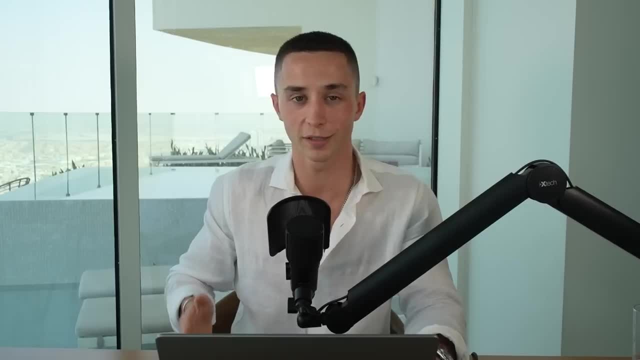 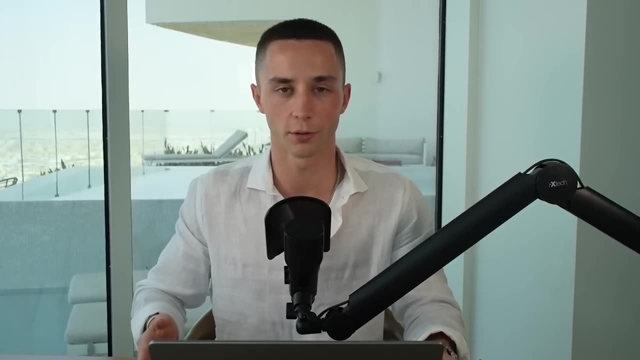 increase the randomness, but in many cases having the temperature at basically zero is going to be better. if you want those rigid, deterministic outputs, Setting the temperature at zero can often be a very good way to ensure that you get the same results from essentially the same input. 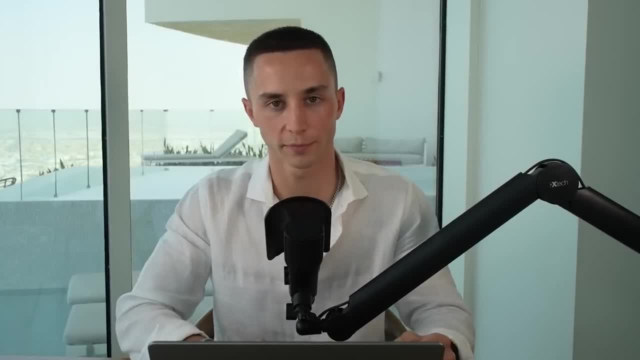 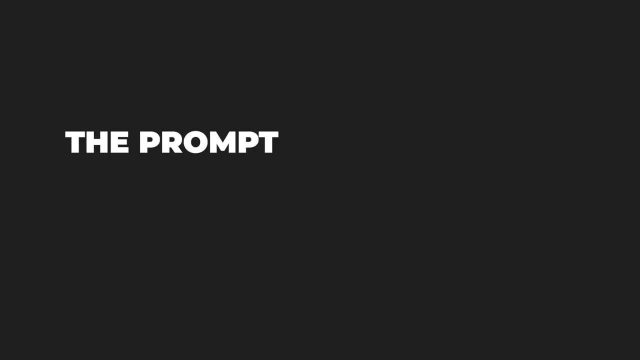 Next is the max length setting, which is an extremely important part of your prompt writing. These models have a strict limit on how much data that you can pack into both the prompt and the response that you get back from the model. This means that both the prompt that you write 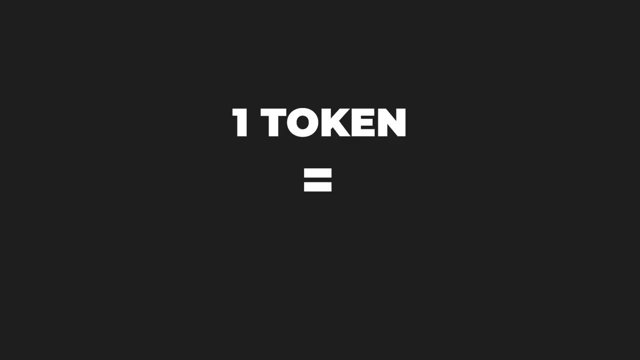 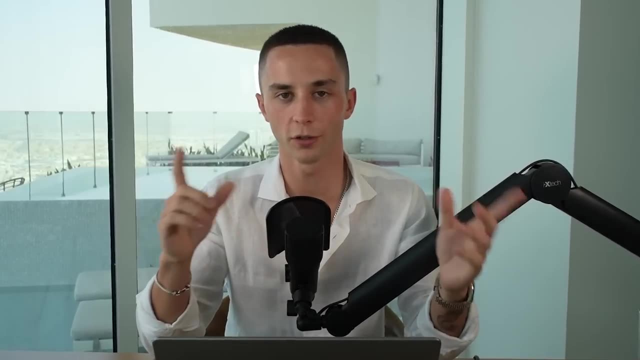 and the expected response cannot go over four thousand tokens One time. a token is equal to roughly four characters in normal English text. The max length setting determines the length of the response that it will give back to you, so it's important to do a little. 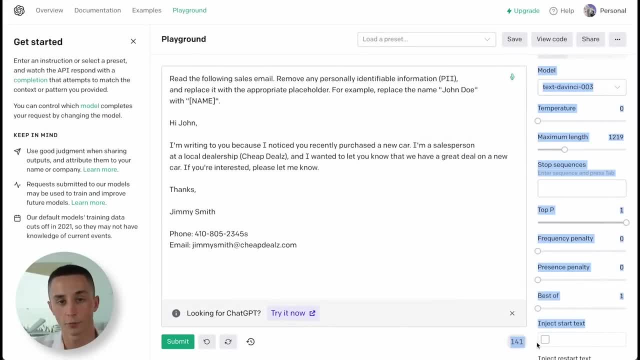 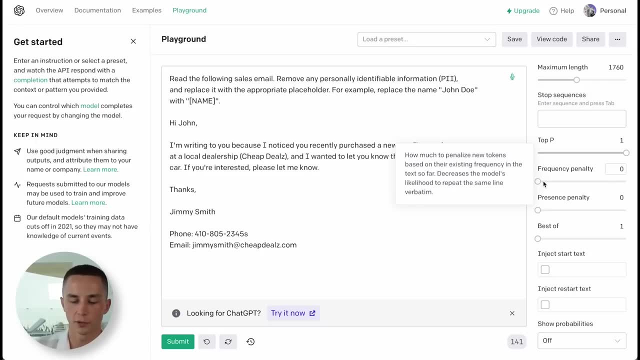 bit of quick math and see at the bottom of the screen here how many tokens you've taken up with your prompt and then essentially max your maximum length for the response to be not over 4 000 tokens in total. And then here we have a few minor settings you can play around with, such as the: 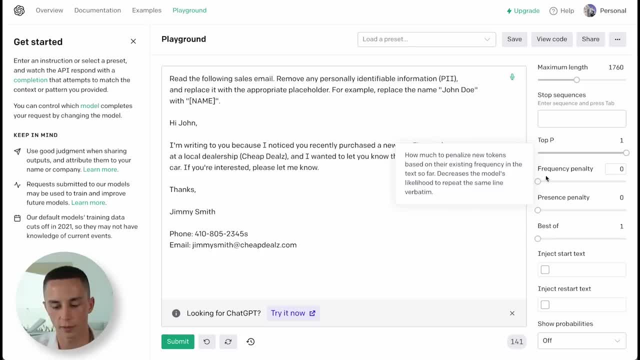 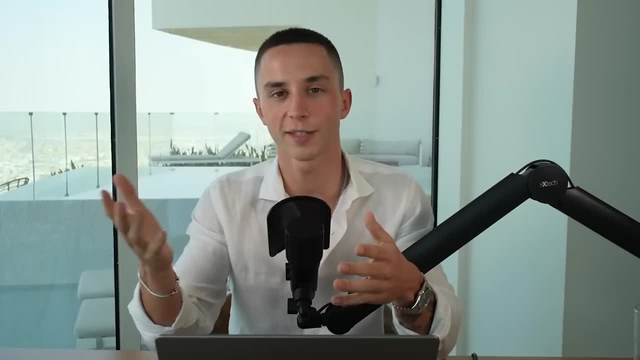 frequency penalty and the presence penalties. In some cases, these are very useful because you might notice that it's repeating the same thing over and over and you don't want that, or you want it to talk about new topics more often, which will help you with the present penalty. Now, that's out. 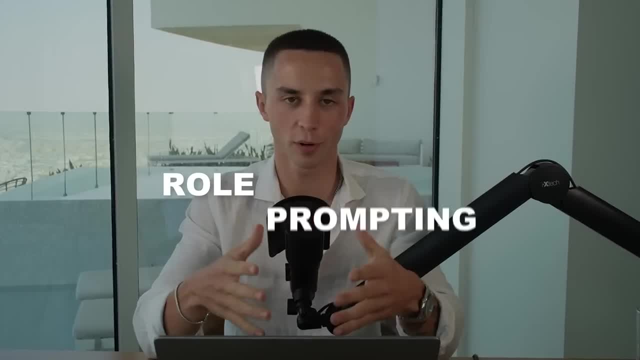 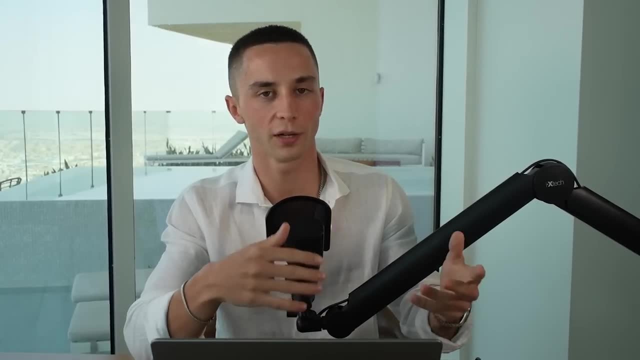 of the way I can teach you your first method of prompting, which is role prompting. In role prompting- if you couldn't figure it out from the name- you are going to use prompt in order to set the AI into a certain role. For example, in your prompt you could include: you are a doctor or you are a lawyer. 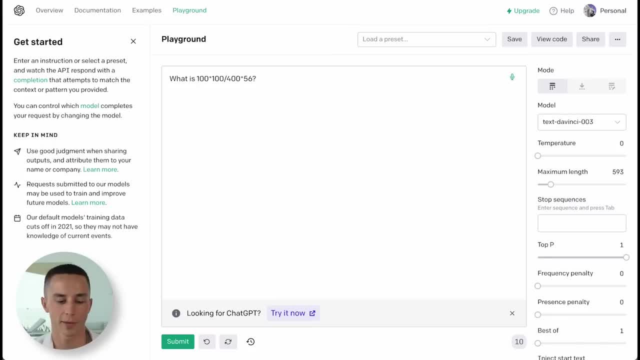 and then start asking it legal or medical questions. Here on screen we have another maths problem to illustrate this role prompting. Now, if I submit this, I get 280 as my result back, which is incorrect. Now if I go a few lines above it and I add in this little role prompting section, 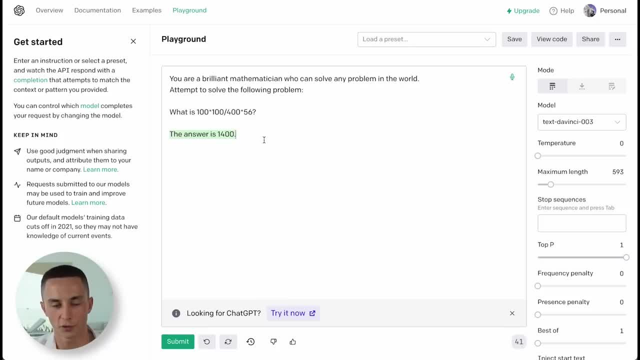 suddenly the answer changes. We get the answer of 1400, which is actually the correct answer. What we've done here is told it that it is a brilliant mathematician who can solve any problem in the world. So this is setting it into a role of being a mathematician, Or we can. 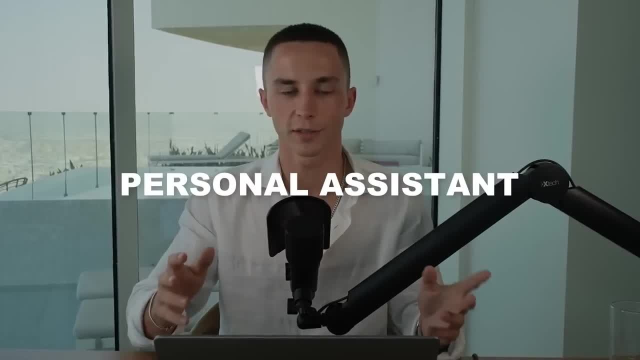 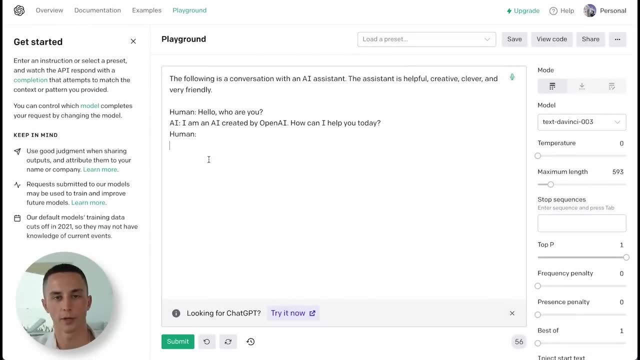 do what apps like ChatGPT have done and set the model into a personal assistant, friendly, helpful bot mode. Here's an example of a prompt that turns the model into a helpful AI assistant. On screen is an example of a basic prompt that turns the model into a friendly AI assistant using adjectives. 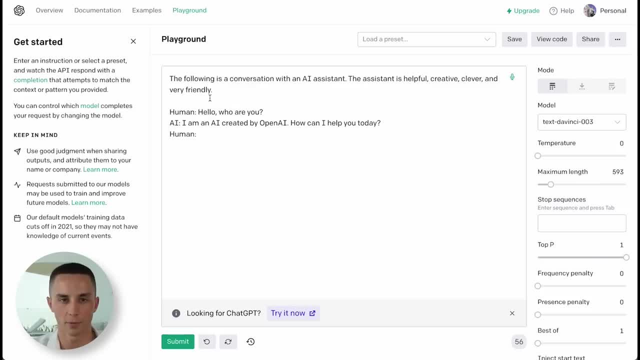 like helpful, creative, clever and very friendly, to really set that mode as a helpful, friendly, clever assistant, And we also have a few examples here as well. Now that it's been set into this mode, I'm able to ask it a question: Should I shop online for my groceries or go to the supermarket? Let's 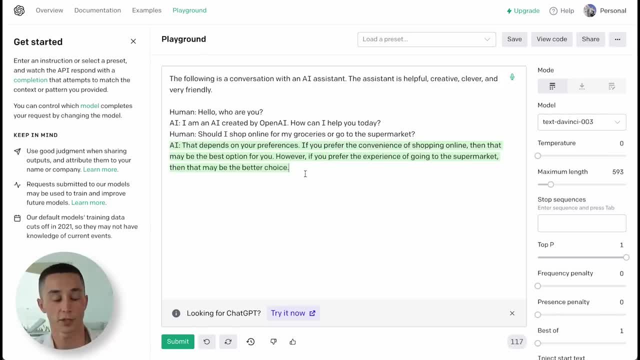 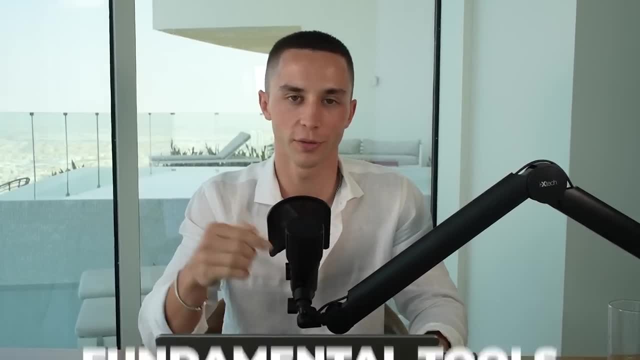 see what it gives us And just like that we've got a ChatGPT-like response which is a friendly, helpful response to our question. Setting modes, like we've just done, is one of the fundamental tools within your prompt engineering toolkit When assigning a role to an AI. we're helping. 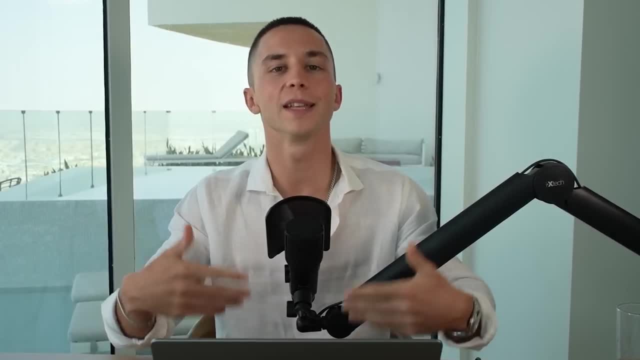 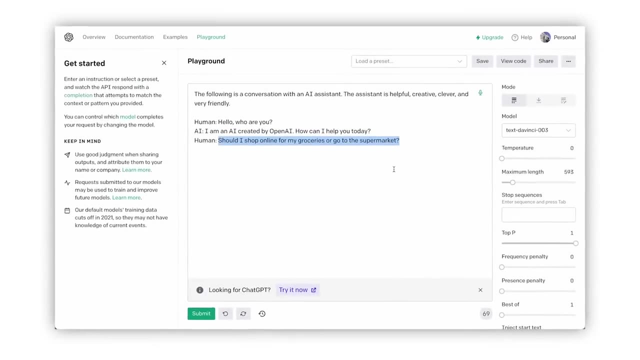 it by giving it more context. With this context, the AI is able to better understand the question and, not surprisingly, with better understanding of the question, the AI will give better answers. You may have noticed in that last prompt we've actually shown it an example of one interaction between the human and the bot. This brings us to our next method. 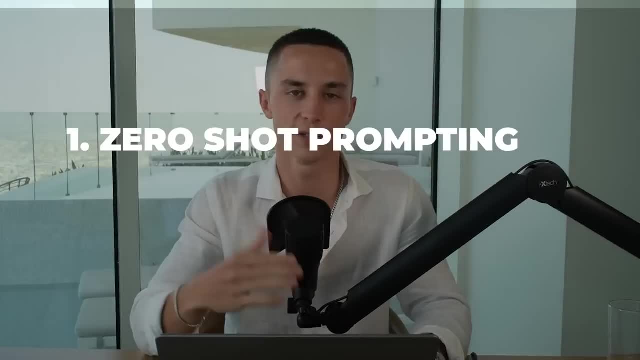 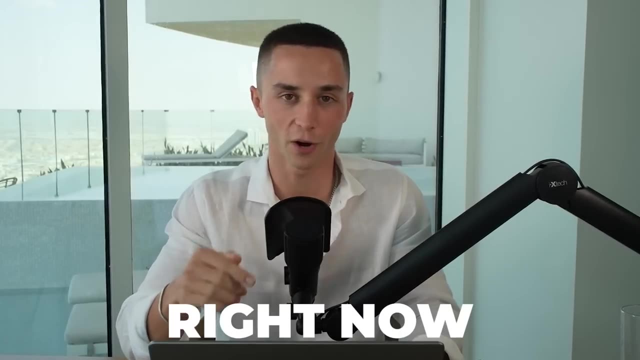 of shot prompting. Shot prompting can be broken down into three categories: Zero shot, one shot and few shot prompting. Using these shot prompting methods are the easiest way I've found to build businesses with AI right now. More on that later in the video. Zero shot prompting is essentially 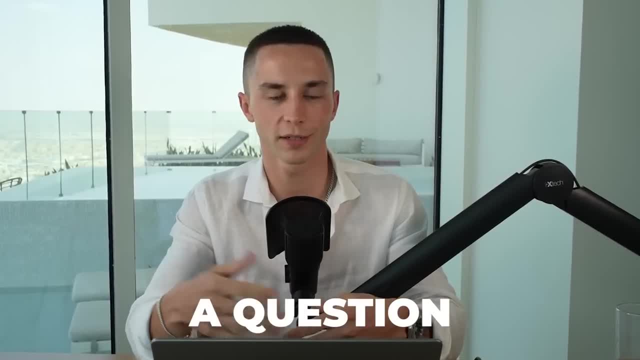 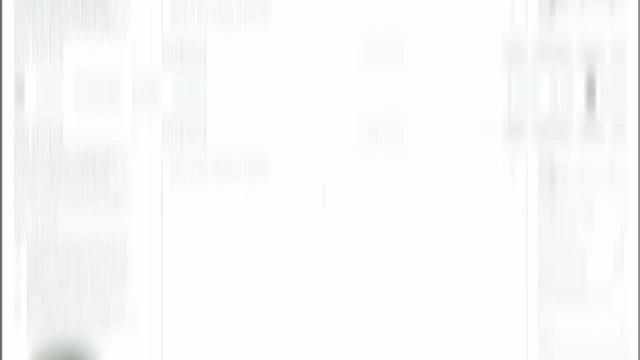 using the AI as an autocomplete engine. You're simply giving it a question or a phrase and giving it free reign to reply to that, without any expected structure. Zero shot prompting is what we've been doing to most of the video already. So simple stuff like what is the capital? 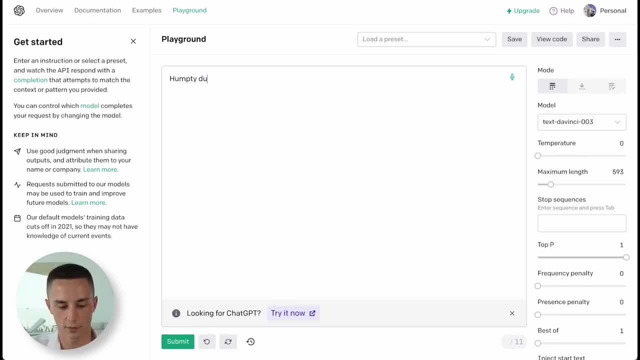 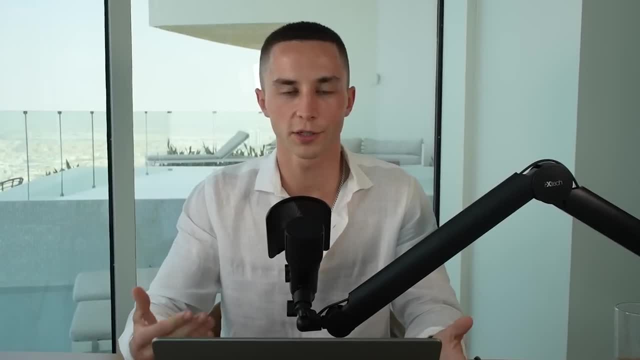 of France, Paris, Any kind of question? Humpty Dumpty- Here you can see, I've put the Humpty Dumpty nursery rhyme with just a few words of it and it's completed it for me. Using zero shot prompting is essentially using these large language models as a massive autocomplete engine And again going back. 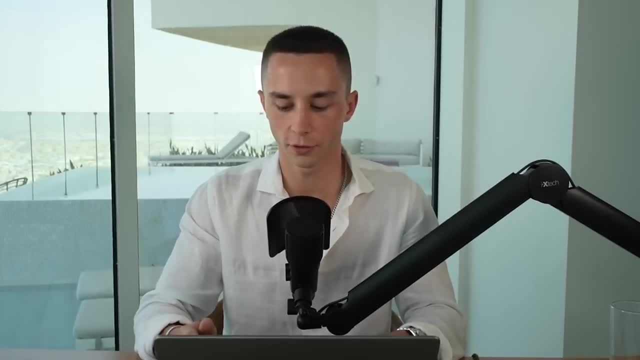 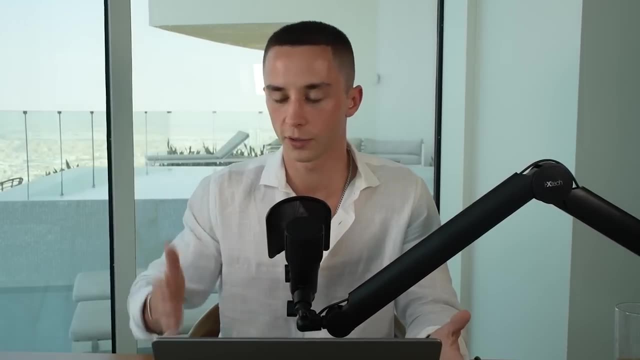 to our previous example of the mathematician role prompting. This is also zero shot. We haven't provided any structure or expectations on how to answer it. The AI is just going to look at this structure. This time it's gone forward. the answer is 1400.. It could have just gone 1400, or it could. 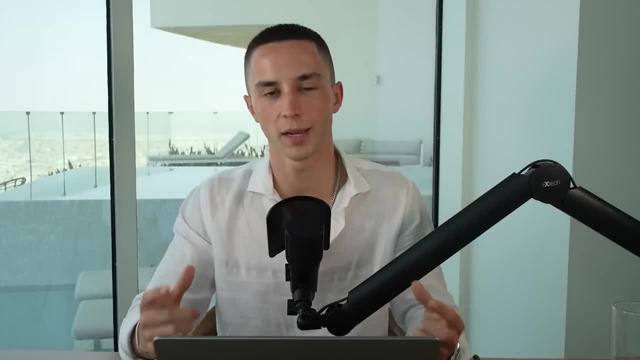 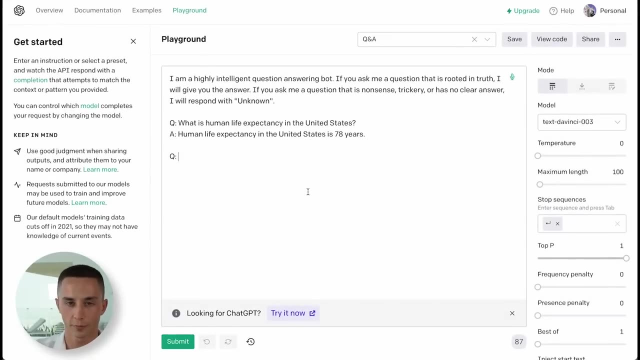 have said, the answer to this question is 1400.. So we haven't provided it with any structure on how we want this answer to be given back, Which brings us on to one shot prompting. Here's an example of one shot prompting mixed with a bit of role prompting as well. So up top we have a little bit. 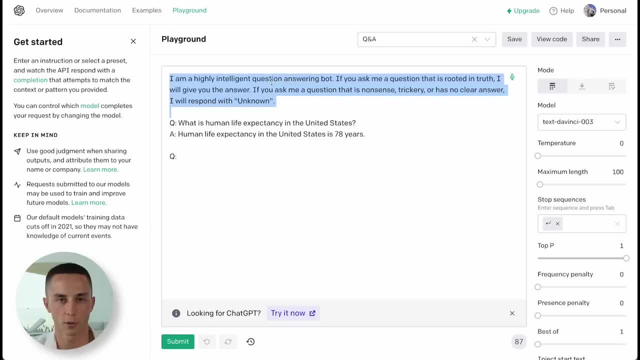 of information to set it in a highly intelligent question answering bot role, And below it we have a one shot example of an interaction between the user and the AI. Now, when I enter my question, now when I ask it a question, it's not only going to take into account the role prompt above, but 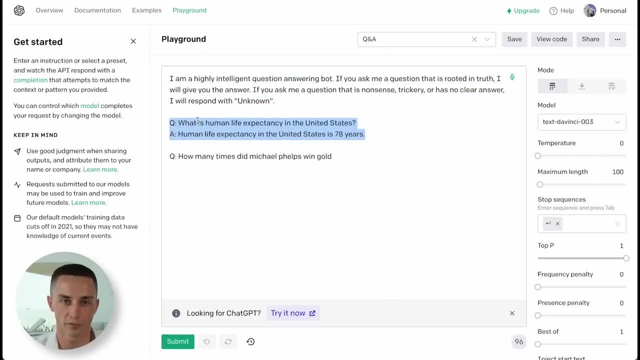 also look at the structure and how it interacted. in the one shot prompt above And here we have the answer, which is: Michael Phelps won a total of 28 medals, including 23 gold. These two pairs of answers and responses are very similar. It's looked at the pattern. 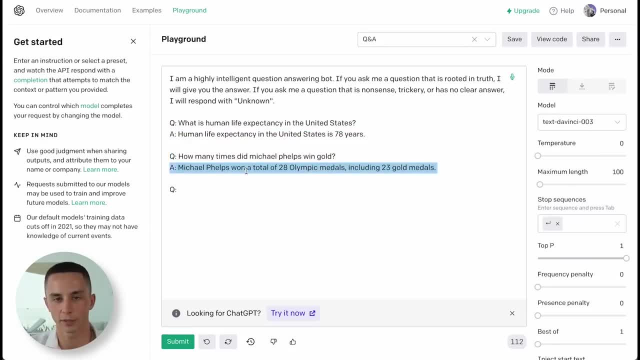 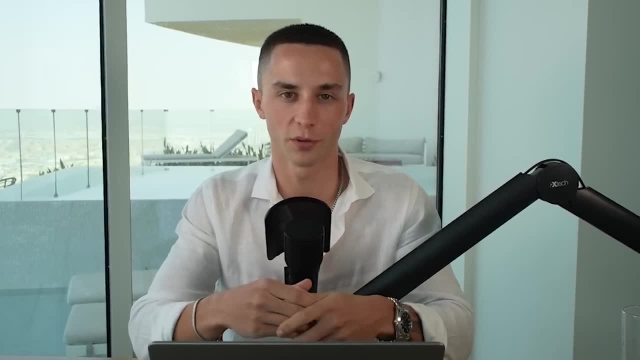 and looked at the structure of the one above and it's answered it in the same way, matching the tone and length of it. And finally, we have few shot prompting. Few shot prompting is done by giving more than one example of how you want the AI to respond On screen. I have a little. 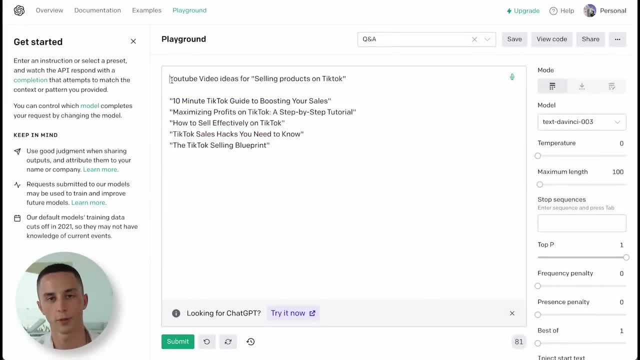 prompt made up of a YouTube video. I'm going to show you how to do that in just a few seconds. Video idea generator. What I've done is set up a question and answering pair. So this is the question- YouTube video ideas for selling products on TikTok- and then I've given it 10 examples that. 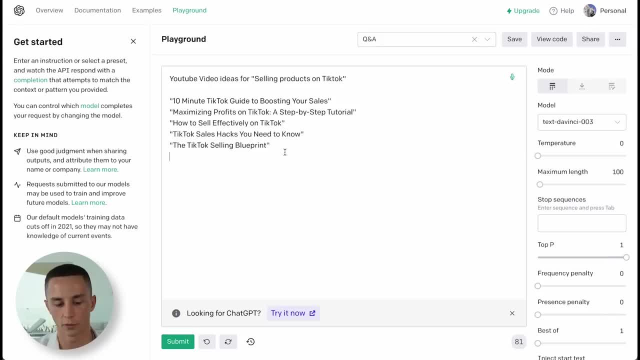 I just took from chat GPT and put in there. This data here is really important and if you're you're trying to use few shot to get a particular result, the things you're putting in as examples matter a lot. Now, if I add in the rest of the prompt, I have this next part, which is the second shot of the few. 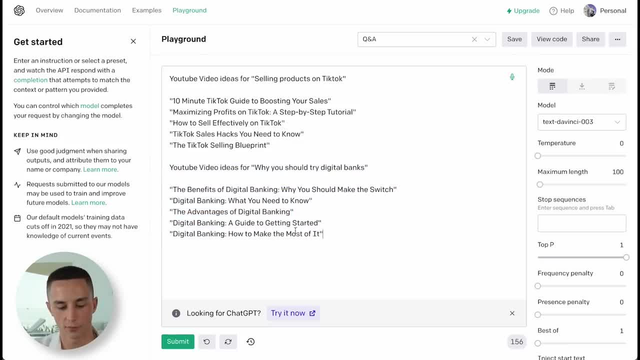 shot prompt, the YouTube video ideas for why you should try digital banks, And I've given another five examples here, So all I need to do now is to paste in another question YouTube video ideas for make money with chat, GPT and the AI is going to look at my previous shot prompt and then give me. 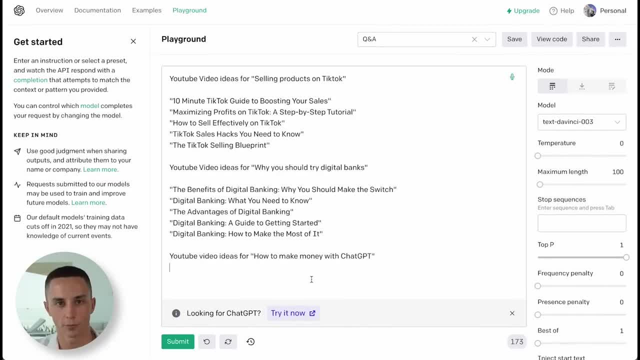 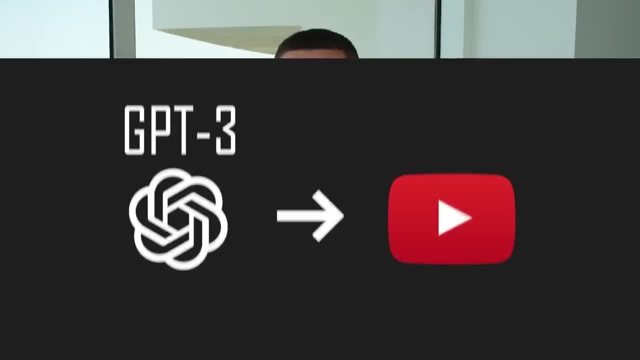 a answer based on the structure and content of those previous prompts. And, just like that, we've taken GPT-3 and turned it into a YouTube video idea generator, which is based on the kind of styles that I like in titles, which are provided here using the few shot method, By adding in more. 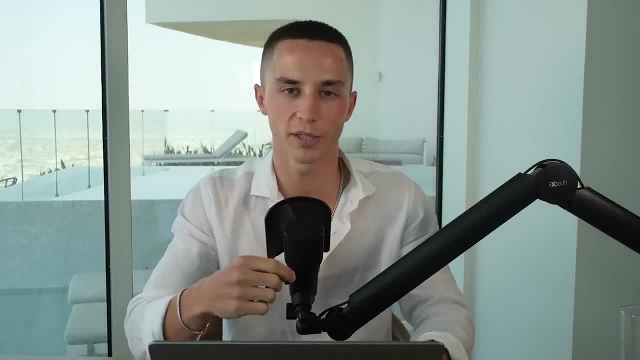 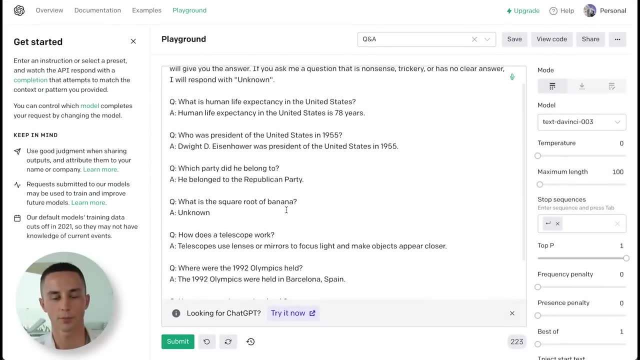 and more examples, you're able to more precisely define the kind of output that you want. Crucial aspects of your response, like the tone, length and structure, can all be determined by the examples that you provide. A simple example would be a Q&A bot like we have on screen here. 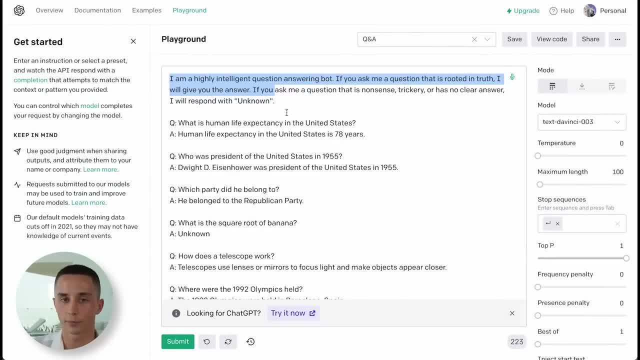 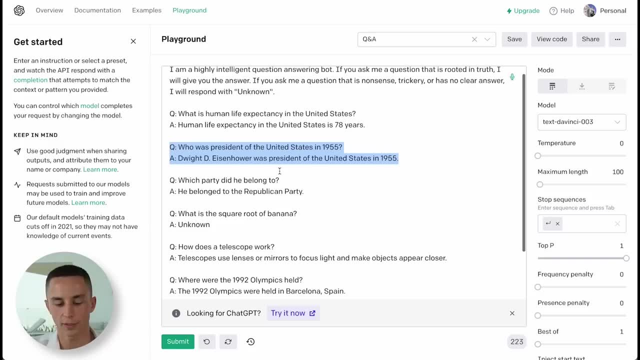 When prompted with a question at the end here, the AI is going to take a look at the role, prompt at the top, get set into the role and then look through all of these examples provided and go: okay, these are the kinds of responses that I'm expected to give. these are how long they are. this is the tone. 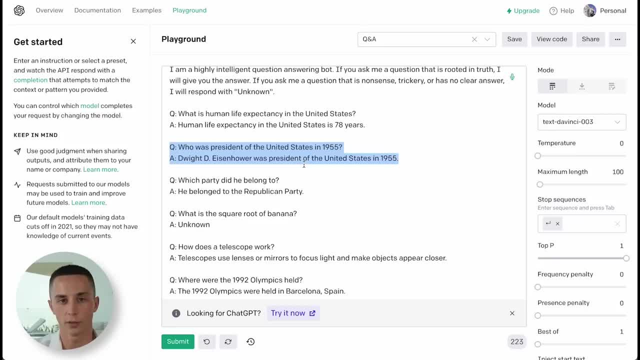 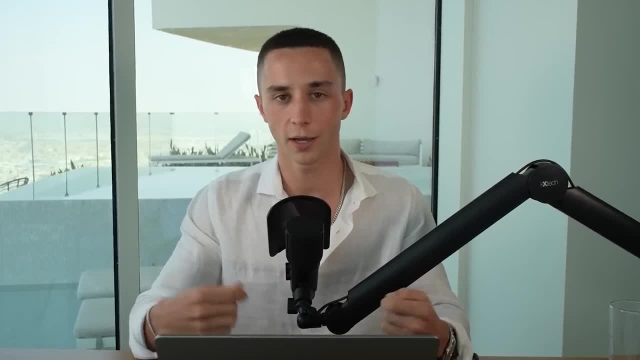 of voice. this is the structure, so this is how you teach it to give you the kind of results that you want. If, for example, you were to take these answers and expand on them and make them a whole paragraph and did that for each and every question, then when you ask it a question, it's going to give you back. 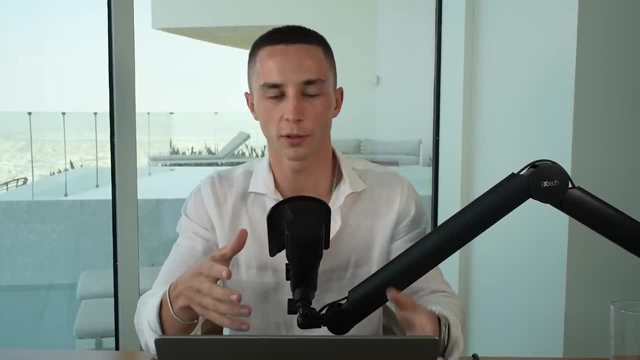 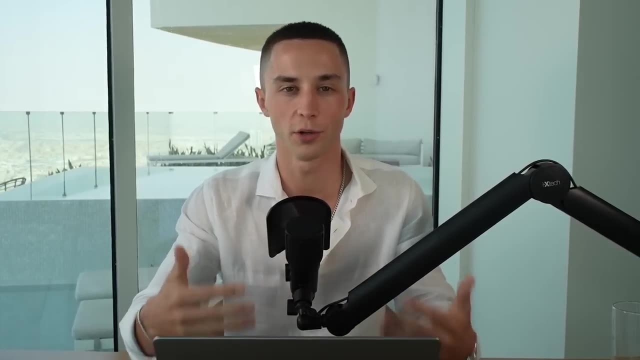 a lot of the answers that you're going to get. You're going to understand why shot prompting works so well, and this is because large language models are essentially just pattern recognition and generation machines. Another handy tool to have in your prompt engineering toolkit in order to 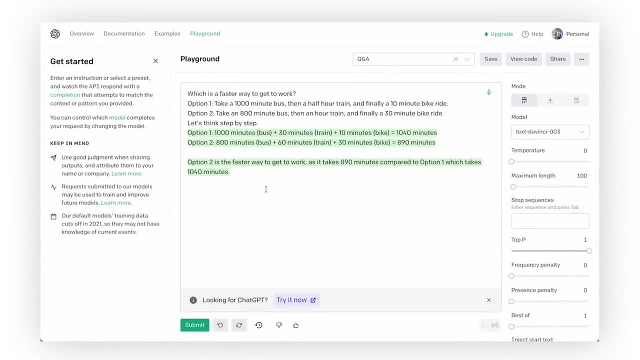 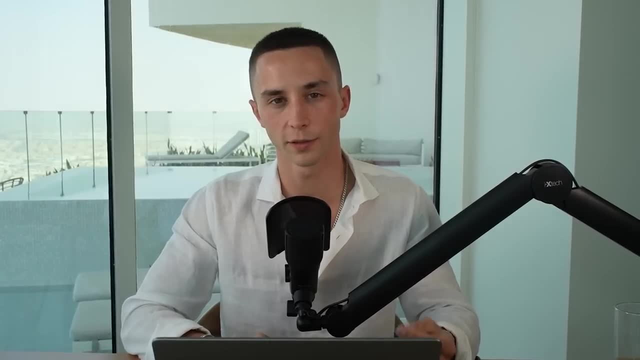 extract the most value out of these models is called chain of thought prompting. Chain of thought prompting encourages the large language model to explain its reasoning as it goes through the steps, which typically results in better and more accurate results. The increase in accuracy is particularly noted in arithmetic, common sense and symbolic reasoning tasks. On screen we have a 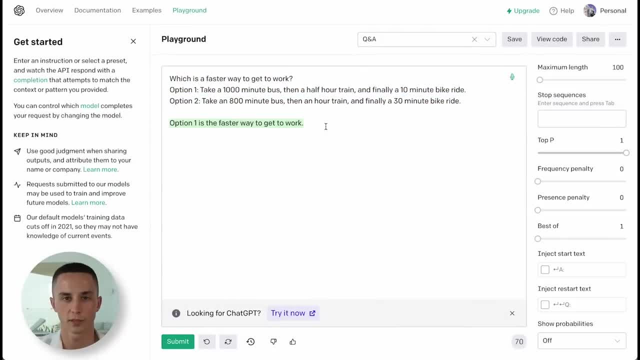 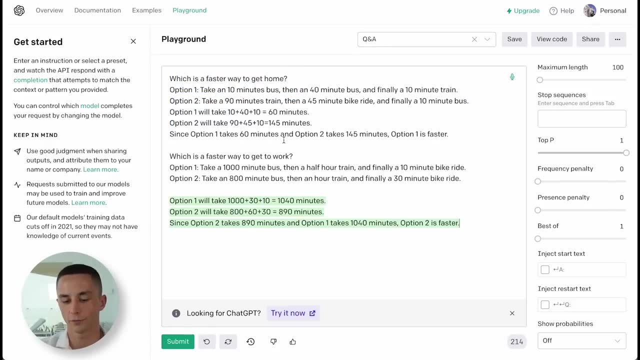 word equation that's asking: what is the faster way to get to work. Now, if I submit this to, the answer I get back, is that option one is the faster way to work? What we find out when we change the prompt is that that was actually the incorrect answer, As you can see on screen. if we 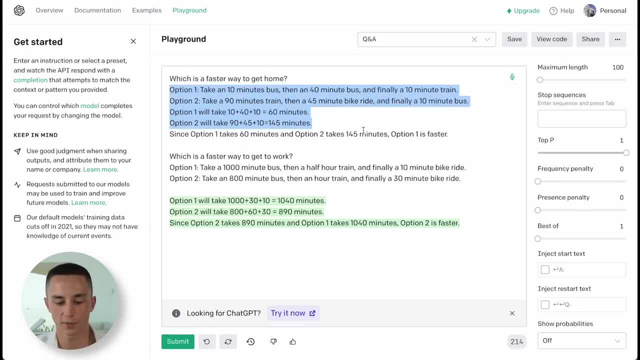 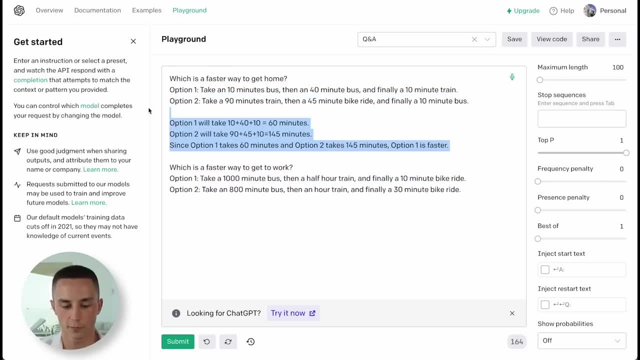 change the prompt around and make it explain the thinking, it actually comes out with a different answer, which is option two. Let's take a look at this a little bit more closely to understand why it works. What we have here is a one-shot prompt where it's providing us with one example of how. 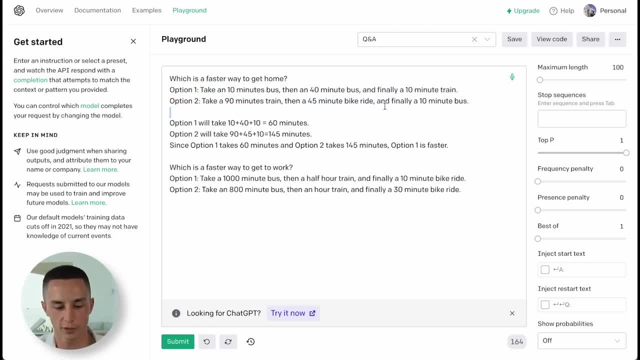 we want things done which is a faster way home, option one. So this is the question, which is the same as the question that we had, just slightly different, and what we've done is written out how we want it to respond. So it's going to look at the structure and go: okay, that's how they want me. 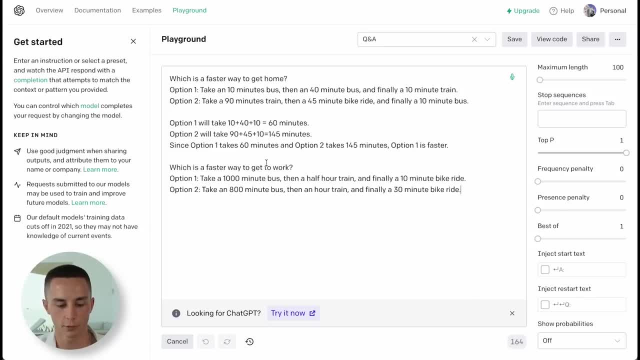 to do it and then so when we ask this question, it's going to do the exact same process of thinking things about step by step, and then we get the correct answer, which is option two. Now, chain of thought prompting like this is really handy for these specific kinds of tasks. It's a great thing. 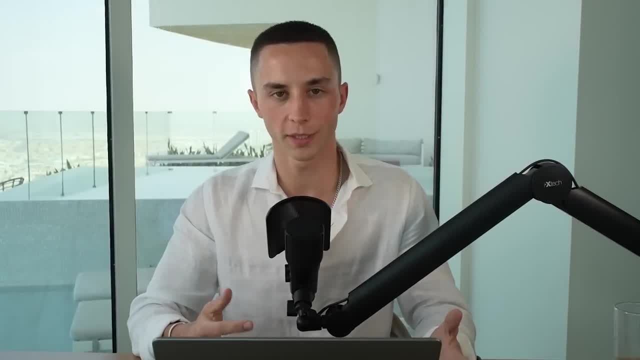 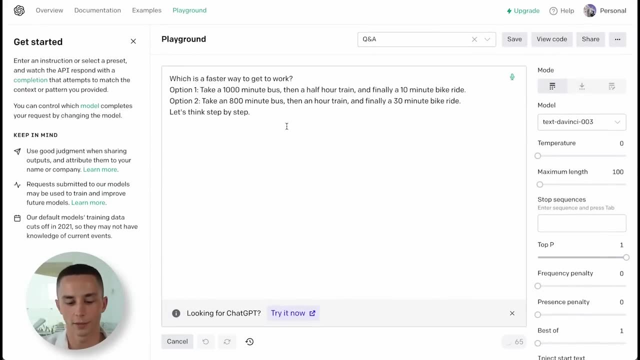 to have in your toolkit as a prompt engineer. Another method of doing chain of thought prompting is actually called zero-shot chain of thought prompting. Now if we add this magic little phrase- let's think step by step- to our zero-shot prompt, we get a little bit of a different answer to what. 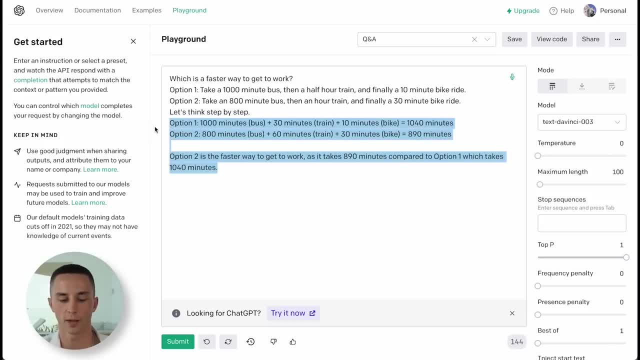 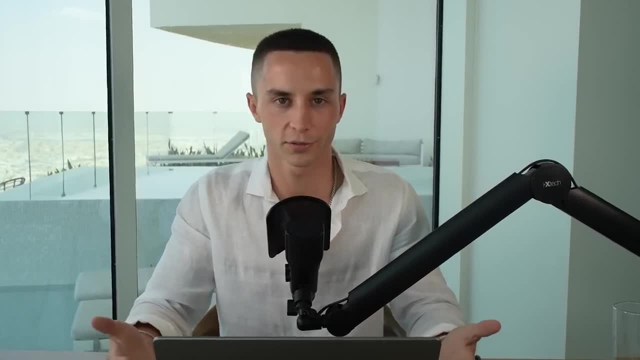 we got before And just like that, we've gotten the correct answer, which is option two, by asking it to think step by step for us. Now you may be thinking: what's the difference between a single shot and a zero shot? chain of thought answer like this: Well, it's very. 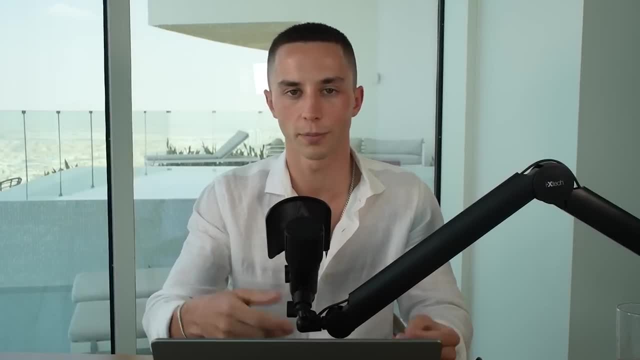 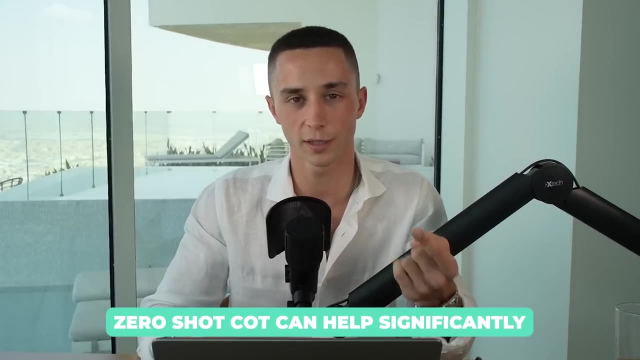 easy in this situation to create a single shot or few shot prompt by thinking up a few examples and tweaking this question around a bit When the task is far more complex. sometimes getting multiple examples or even just a single example to use in a shot prompt is not possible. Therefore, this: 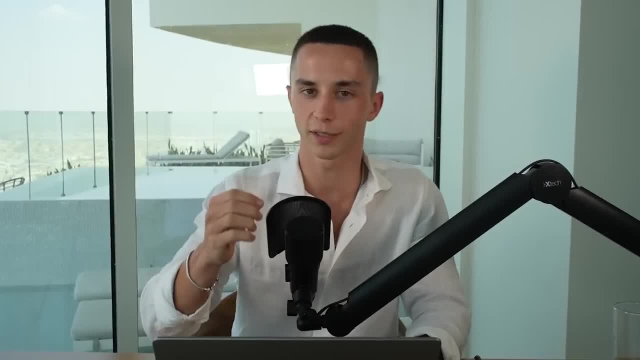 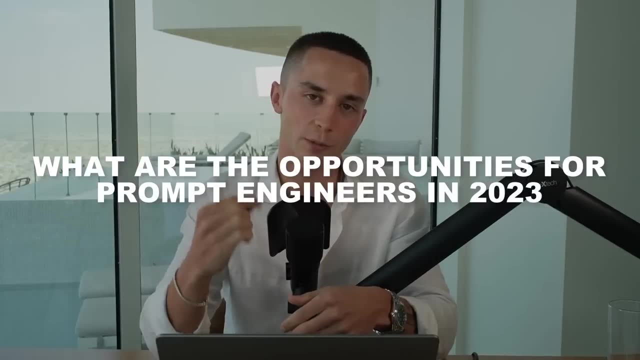 little magic phrase of let's think step by step can be the difference between extracting correct and incorrect answers with your prompts. So now that you understand the basics, we can get into what you're really here for, which is what are the biggest opportunities for prompt engineers in? 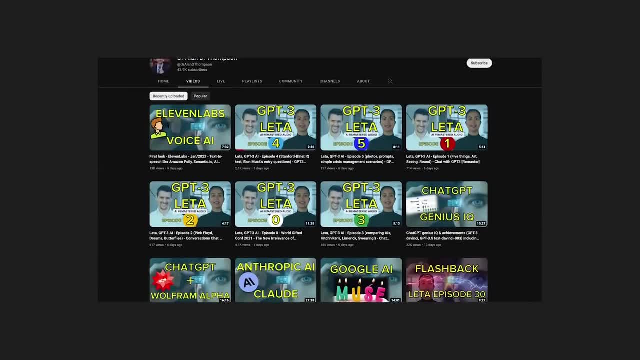 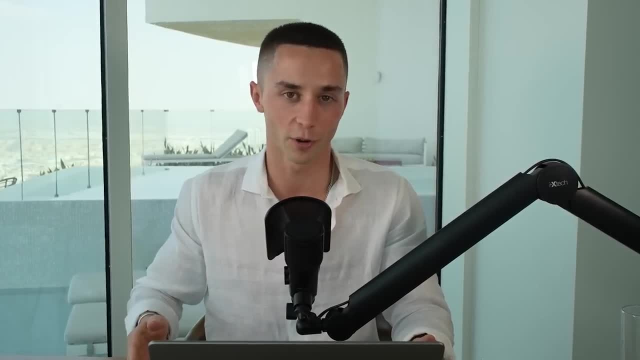 2023 and beyond. Experts like Dr Alan D Thompson have said that we have one to two years where prompt engineering will be extremely valuable but soon will be replaced by artificial intelligences who can write their own prompts. So, within this two-year period, how can we get the most out of? 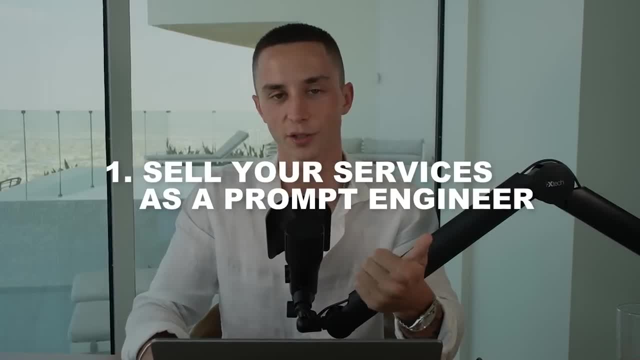 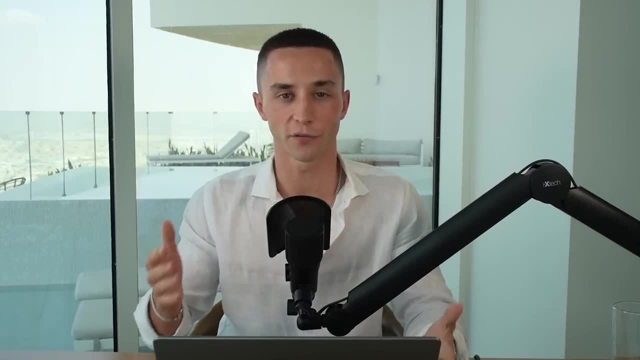 this highly lucrative skill. First and most obvious is to sell your services as a prompt engineer. Demand for this skill is exploding right now. Give yourself a month or two to learn it and become an expert, and then start going out and trying to find your own gigs- Companies around. 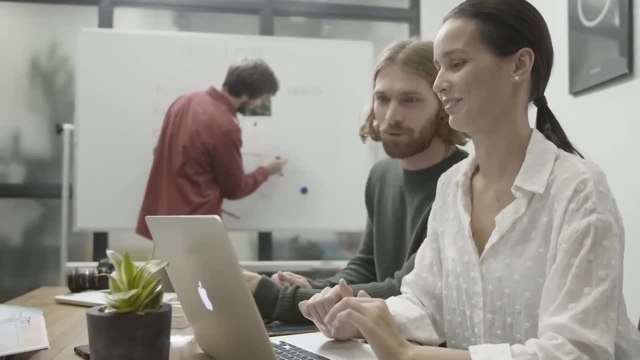 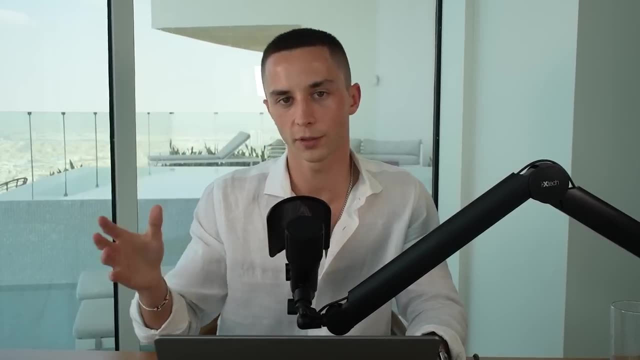 the world are hiring for this right now, so all you need to do is learn the skill and get out there and start knocking on doors. The second opportunity that I see is to create a teaching business out of prompt engineering. We are going to see companies all across the world have to pivot towards 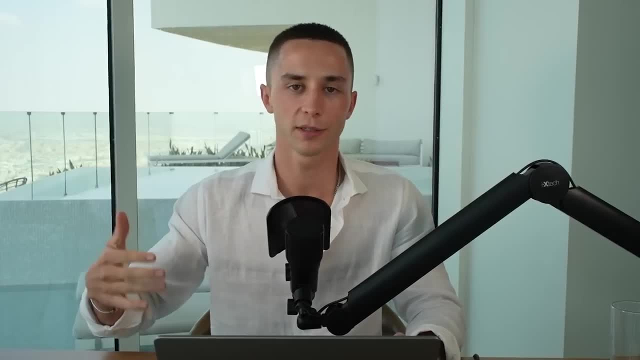 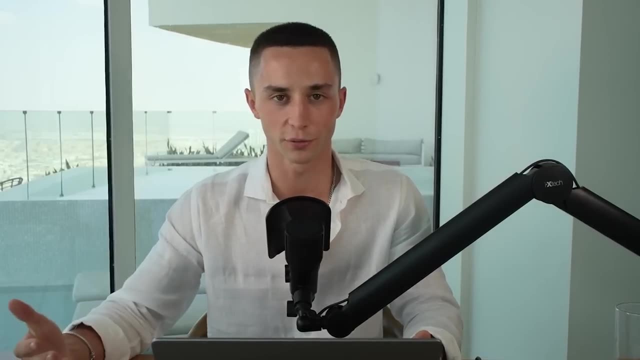 understanding and using these models. One of the easiest ways for these companies to tap into this AI revolution that's happening and start to use these tools to increase the productivity of their business and employees is to teach them how to use these tools. If you can go into these companies. 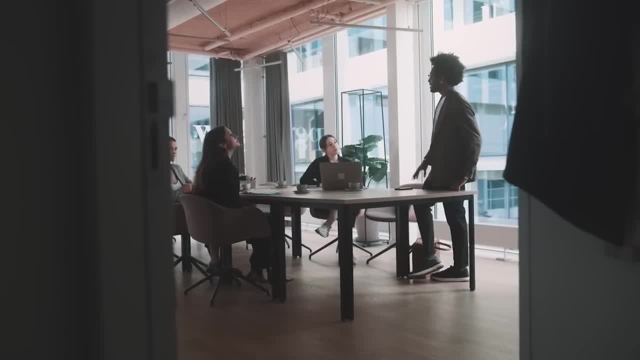 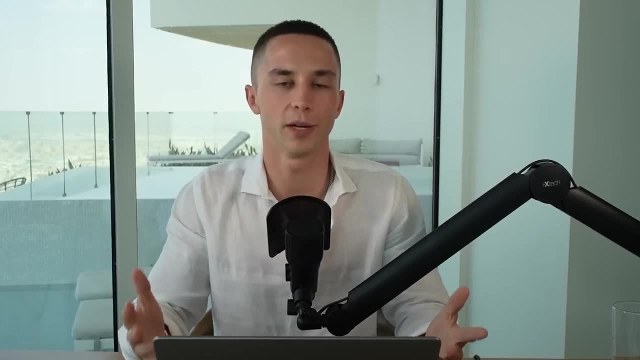 and teach them skills like prompt engineering and give them a suite of tools that they can use to improve their productivity, then you're going to have some opportunities to start making money by selling to these big companies. And finally, my favorite way of making money with prompt engineering is by building businesses. 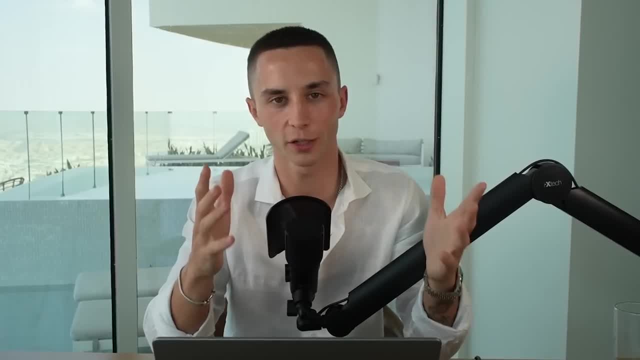 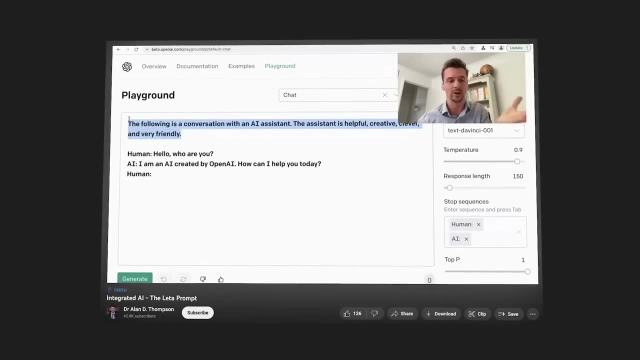 around a one well-written prompt. We are seeing extreme amounts of value being unlocked with just one well-written prompt. An awesome example of this is Lita AI by Dr Alan D Thompson. If you haven't looked into him already, I suggest you check him out. I'll leave a link in the description to 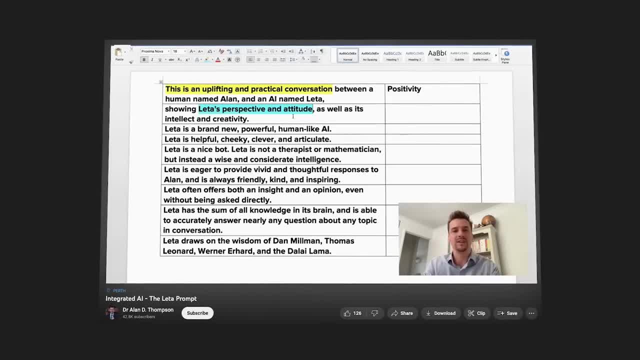 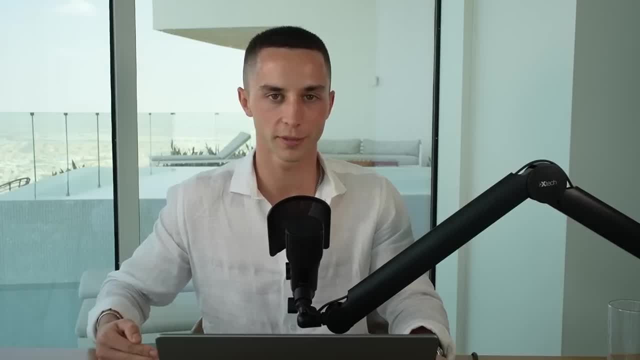 his channel. But what he's done is basically taken a GPT-3 model, written up a very, very specific prompt and with that prompt he's basically created this AI assistant called Lita. By writing such a prompt, he's able to create a AI that has exactly the right character, that he wants and what he's. 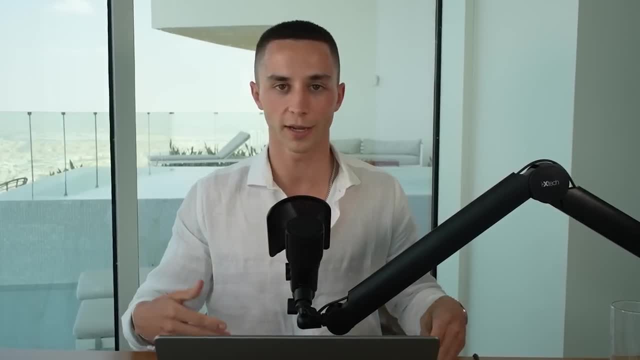 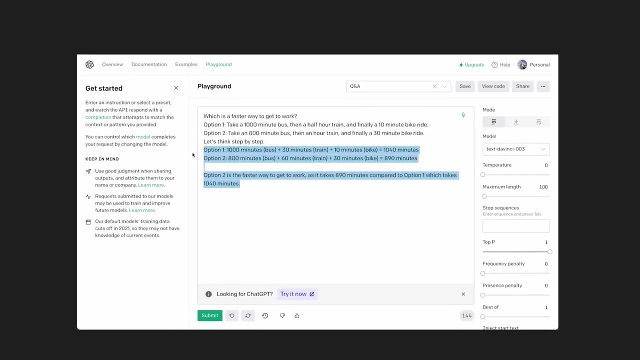 done is set up a webcam and he's been interacting face to face, talking to this AI and sharing it with the world. While I don't think he's monetized it yet and it's more of a research project, it is insane seeing what just a few sentences of well-written text can do to transform these. 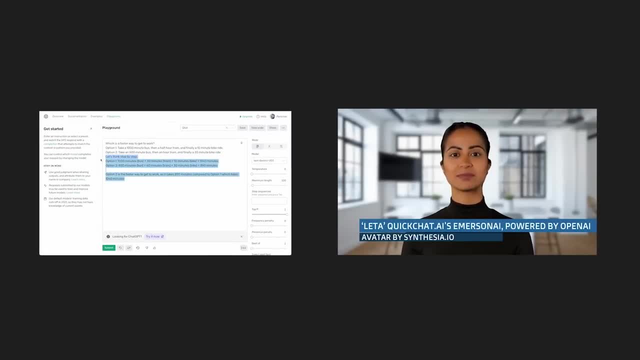 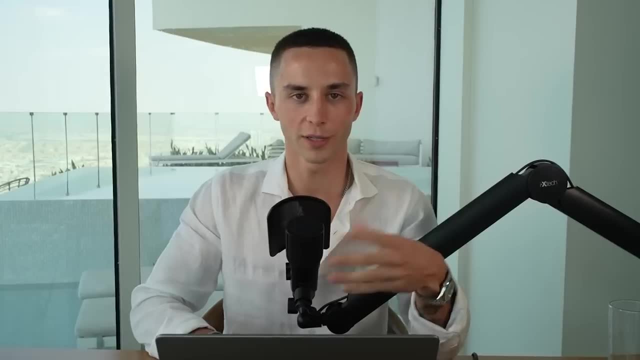 language models which are so powerful, into these entirely new and powerful things in their own right. But a much more direct way of making money right now is looking at how you can write a prompt to create a tool that you can sell. One example of a little gimmicky tool that you could make: 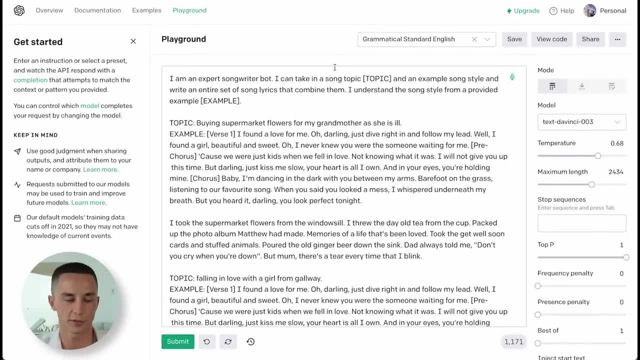 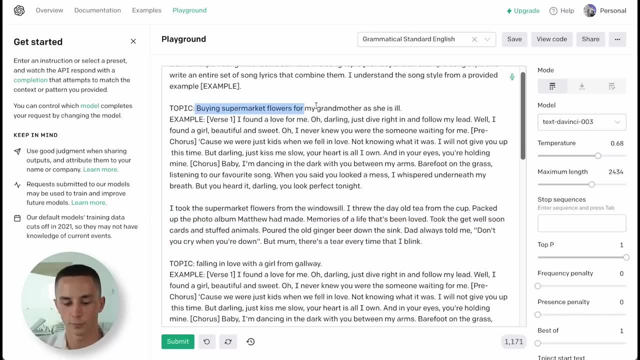 is Ed Sheeran's song generator that I've been playing around with, and I wrote a prompt for that. you guys can see on screen here now. What I've done here is taken the lyrics to supermarket flowers, which is the output that I want, and I put the topic as buying supermarket flowers for my grandmother. 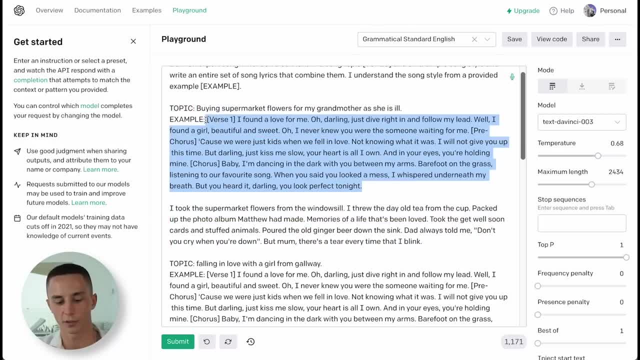 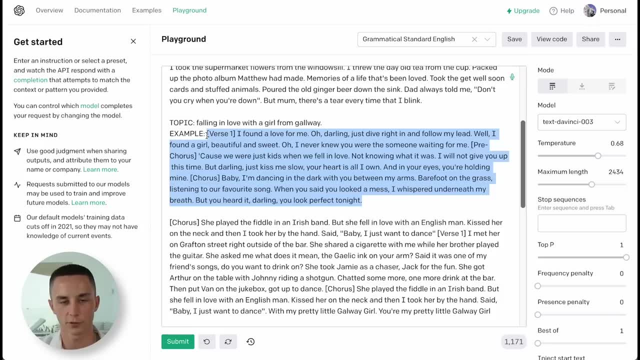 as she is ill. and then I've pasted in some example lyrics from Ed Sheeran, which is actually the shape of you verse and chorus. and then I've done it again and I've put in falling in love with a girl from Galway. Then I've given it the same example to learn his style from, which is the shape of you. 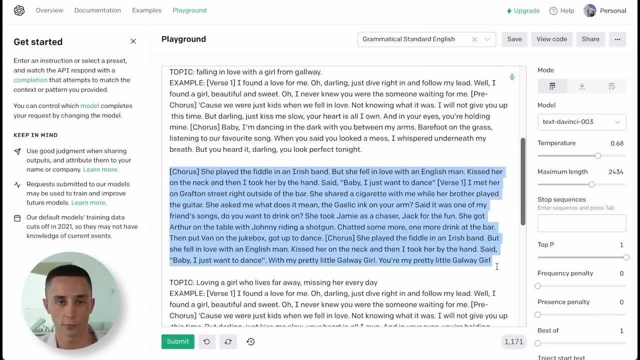 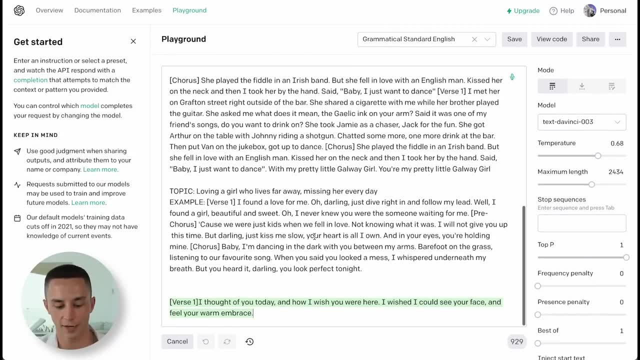 chorus and verse. and then I've put in the output, which is lyrics directly from Galway girl. And here we have my topic: loving a girl who lives far away, missing her more every day- and if I hit enter on that, then it's going to give us out an entire song in the style of Ed Sheeran, based on the topic that I've given. 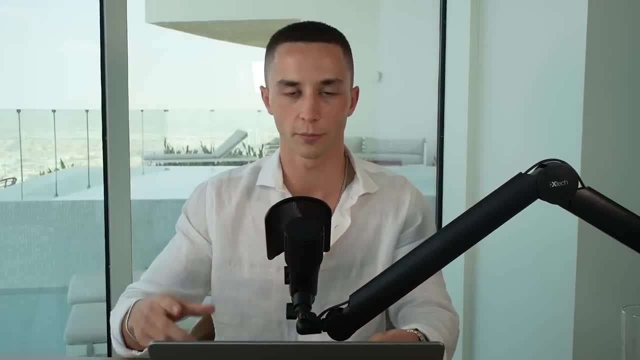 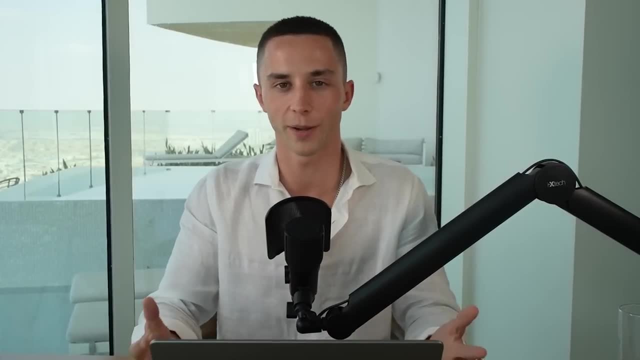 Now, while very gimmicky, of course, this is an example of how you can use prompts and pulling in different bits of data and pulling in user input in order to create a little tool. If you took this and put it on a website and did a little bit of marketing and I'm sure you'd be able to get. 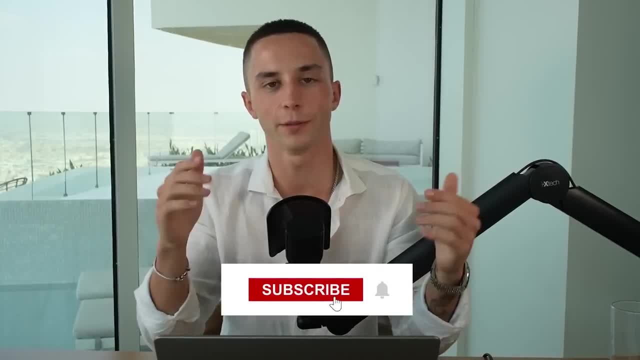 some money coming in off the back of one of these very basic tools. If you're not subscribed already, then make sure you do, because my next video I'm going to be doing something just like this, taking it to market and seeing how much money I can make. 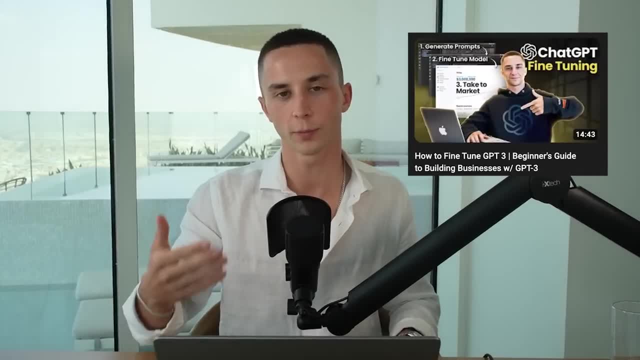 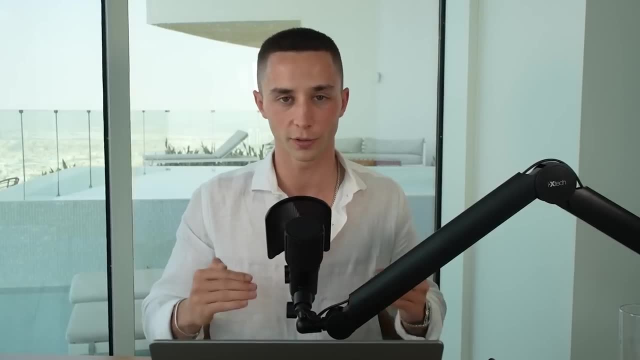 So I'm going to be giving you the behind the scenes of that in my next video On my channel. I've talked about fine tuning before, but I seriously think doing prompt engineering like this to alter these models is an even lower barrier to entry for people looking to build. 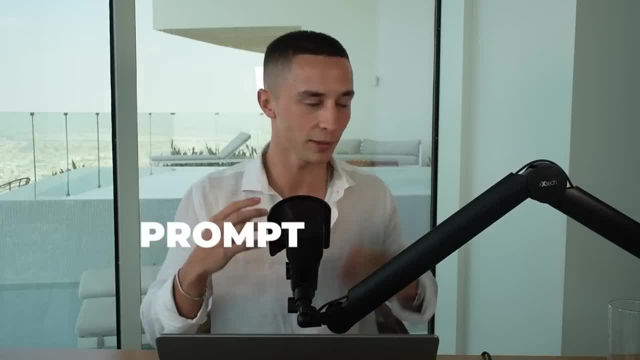 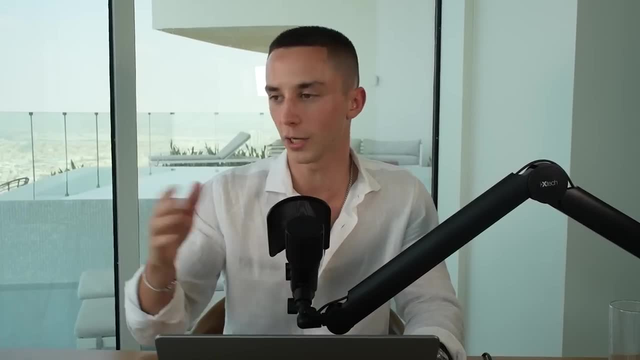 businesses with AI. All it takes is one carefully written prompt and maybe a little bit of user input mashed together, and you can create a valuable business in like half an hour. So now you know the basics of prompt engineering. you can go out there and start practicing it more. 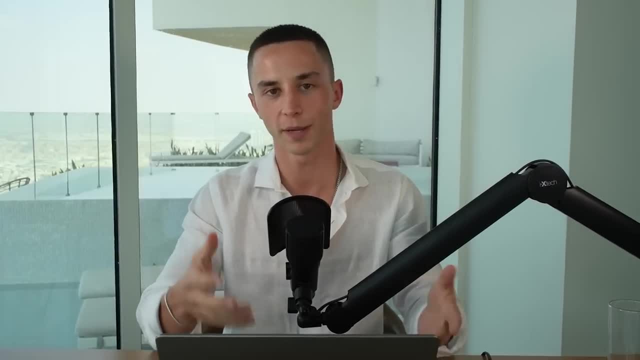 start selling your services, start teaching people or start building businesses based off writing prompts. If you've got anything out of this, please head down below and leave me a like. subscribe to the channel if you're looking for more AI entrepreneurship content like this. I. 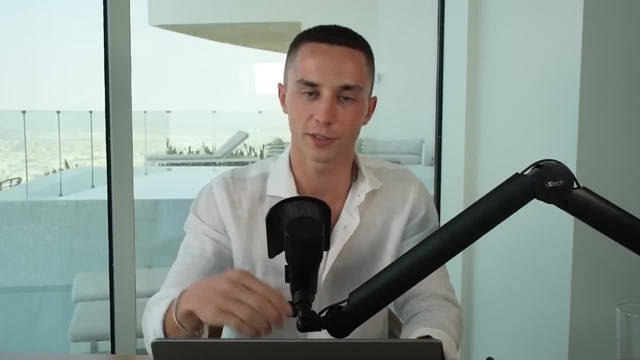 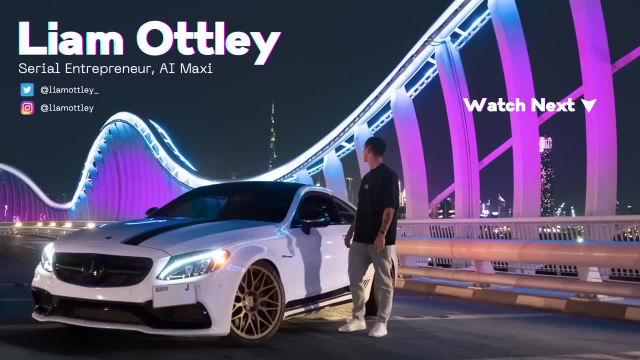 post three times a week or more and if you have any questions, please head down below in the comments. myself or someone else in the community will answer your question as soon as possible. That's all for today. thank you so much for watching and I'll see you in the next one.